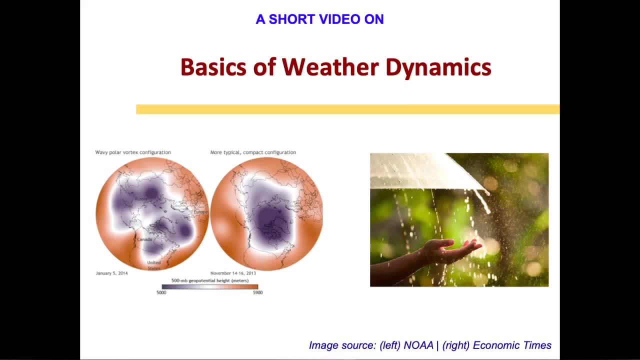 I thought I will do a different thing today, wherein I'll just present to you some basic aspects of weather dynamics, Not talking about one single aspect, but multiple aspects, and mostly from a basic viewpoint, so that this can actually probably lay a platform for people who are interested in weather systems and weather dynamics. 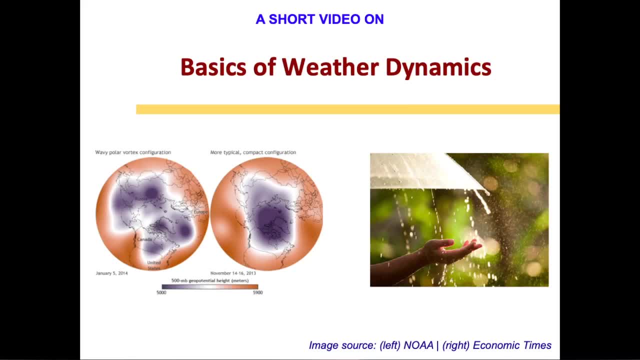 To take this up as a career or also to learn more about them and get intrigued. Okay, so that is the idea. So this is going to be a slightly longish video, but, given the aspects that we are going to cover, it is not a very long video because, as you will see, different modules will be covered. 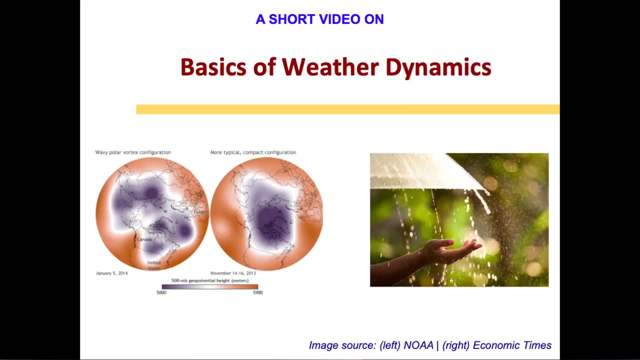 Maybe this is going to be a 30 minute video is what I feel, And I just want to put a disclaimer that whatever I am presenting in this video Is only the tip of the iceberg as far as the dynamics are concerned. Okay, and there is a lot, lot and lot to learn. 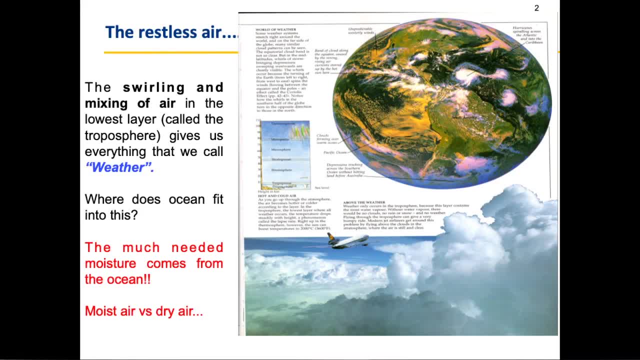 Alright, so let us start. As we all know, the reason we have weather is because the air is restless. It is never in a state of rest, It is always moving, And that is why we have something known as weather, And in all of these, usually whenever we talk about rain or systems. 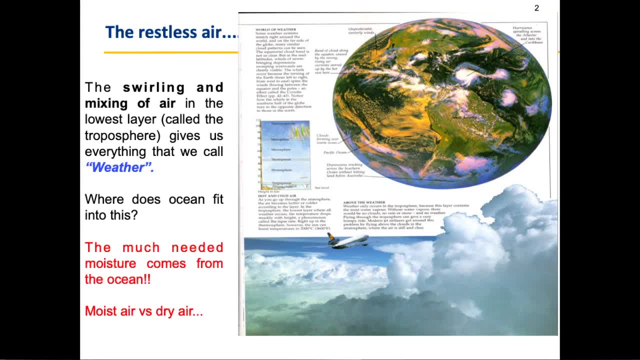 They are always in the atmosphere, right, They always move in the atmosphere, And that is how we get rain. When you talk about clouds, when you talk about cyclones, everything is in the atmosphere, But ocean importance is seldom underappreciated, because the much needed moisture comes from the ocean. 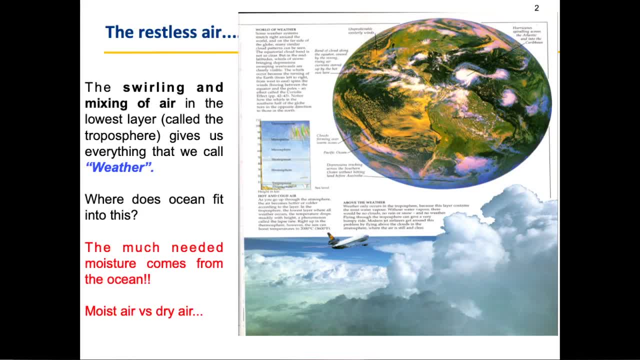 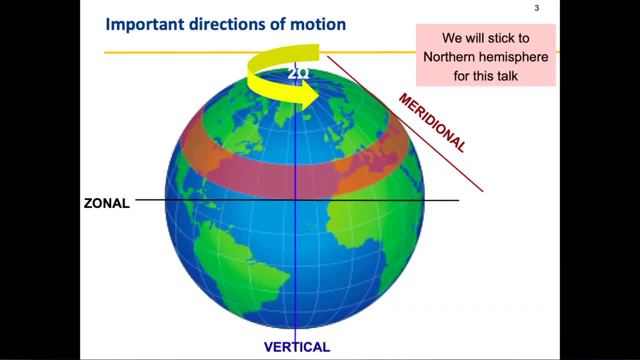 Unless and until you have moisture and dry air interacting, you will not have any systems that form Okay. so the role of ocean is very, very crucial in all of this. So, before I get into a little bit of, So, before I get into a little bit of, 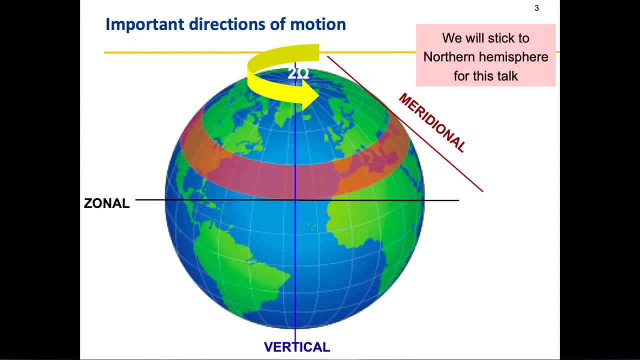 So, before I get into a little bit of for our technicalities, Let us lay a platform for what are the important directions of motion as far as our system or at this concern. So on a rotating frame of reference such as the Earth, which is critical in shape, 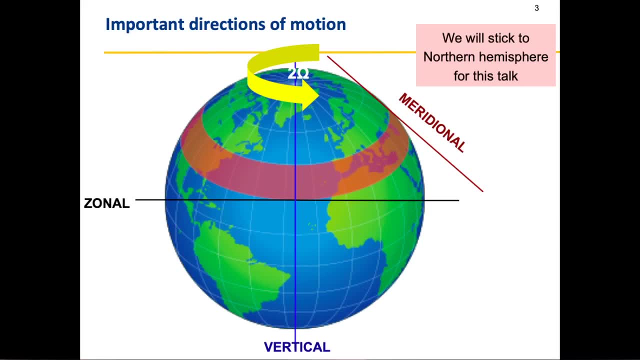 you have three important motions which are zonal, which is east to west or west to east, and then you have the meridional, which is north to south or south to north, and you have a vertical direction which is looking up above the ground. okay, so these are three major directions of motion and of 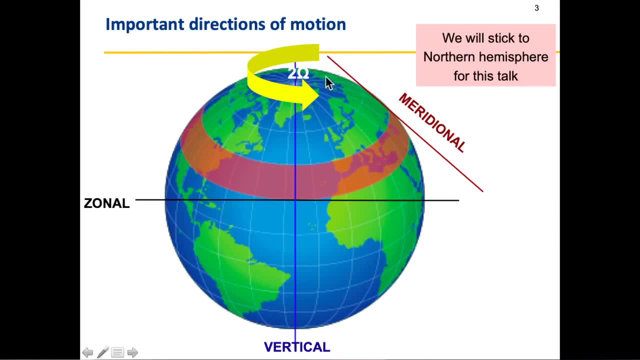 course, the two omega that i have shown here is basically the coriolis effect, because the earth is rotating. so for this particular talk or the video, i will only stick to the northern hemisphere, but similar as similar things happen in the southern hemisphere as well. the reason: 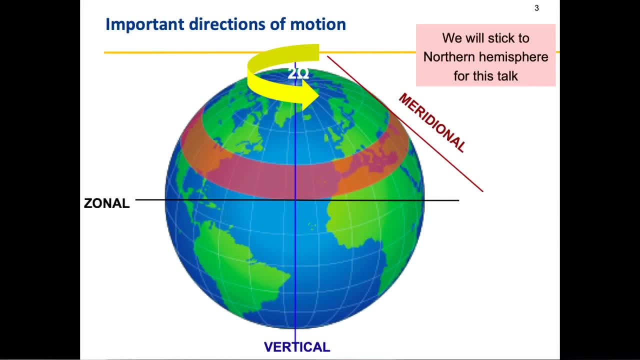 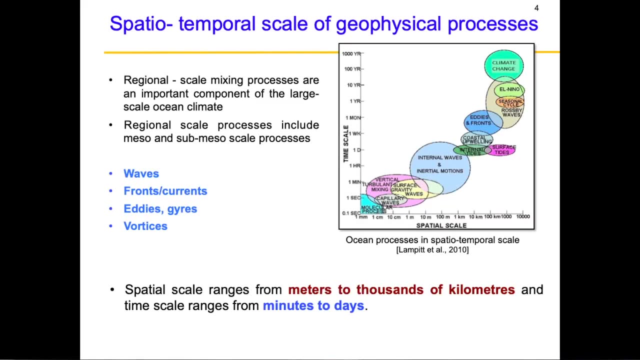 i am sticking to northern hemisphere is because you have more landmass in the northern hemisphere, so that's the only reason i am sticking to northern hemisphere. so on a spatio-temporal scale, if you try to really relate the processes that happen in both ocean or atmosphere, then 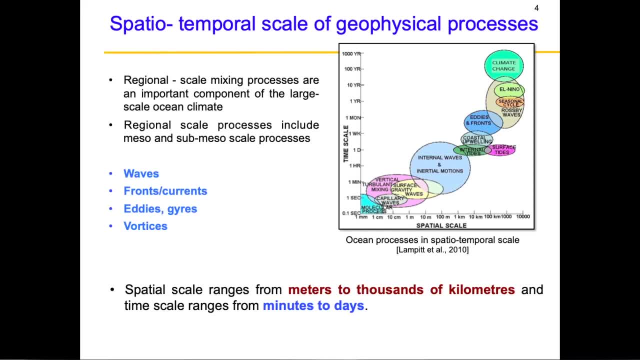 you actually have multiple scales, all right, and this is what makes weather a very, very complex topic. so you, if you have time scale on the y-axis and the spatial scale on the x-axis, then you have systems that can vary from as small as one millimeter or hundred. 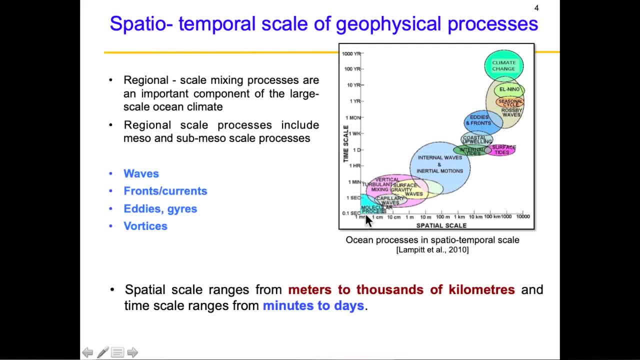 uh microns, which is as small as the width of your hair and systems, can then go as large as thousand kilometer, which is your cases, like waves which are kelvin waves or rosby waves, which are like hundreds or thousands of kilometer long, and that is the spatial scale that we are talking about. and 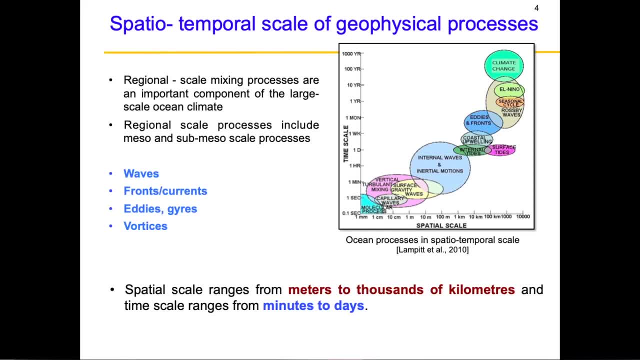 the temporal scale is anything: a process that can last for 0.1 second and a process that can last for thousands, hundreds or thousands of years, like climate change. so this is the spectrum of scales that we have to capture to really really pin down weather and, as you know, 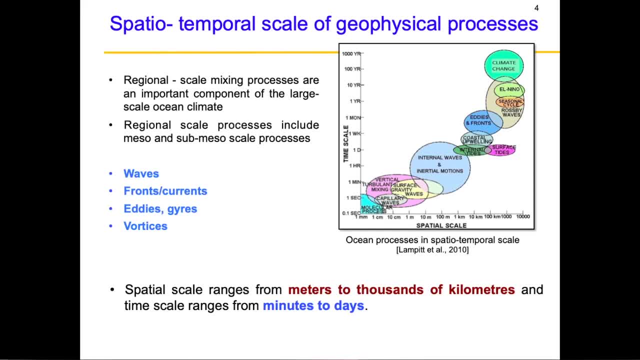 models don't have this capability, because our best capability is 10 kilometers. is the spatial resolution and of the order of six hours? is where is, where is? is how we can uh on a time scale? is where is the feature that we can capture, so anything which is less than, let us say, six hours? 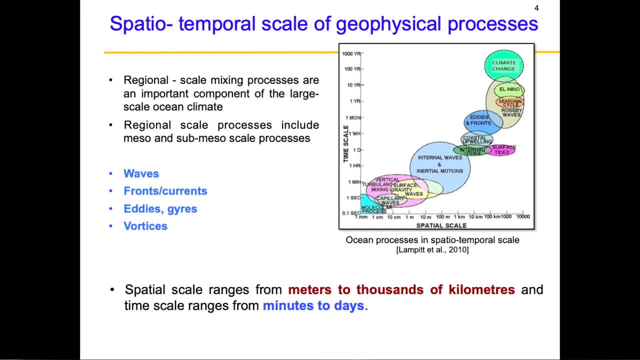 it's very difficult to capture. so that's the reason: clouds, which are of order of three hours, are very hard to capture at that moment, as also very hard to capture. so another famous thing, quote exists that even if you, even if you move your head, where in your hair is hundred microns, which is 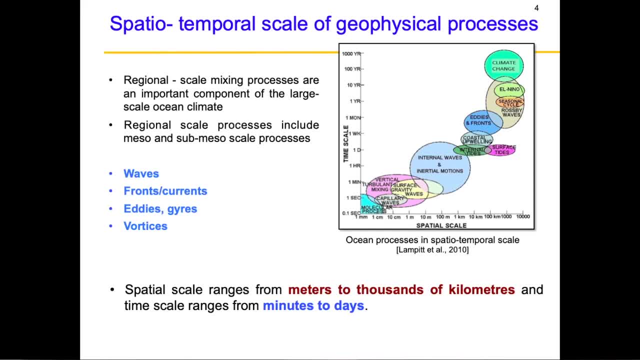 just flapping and that is going to create turbulence or an eddy in atmosphere and that has a capability to change anything in the other part of the world. let us say you are sitting in India and you are just waving your hand or moving your head. that can change the weather in Africa or America or any. 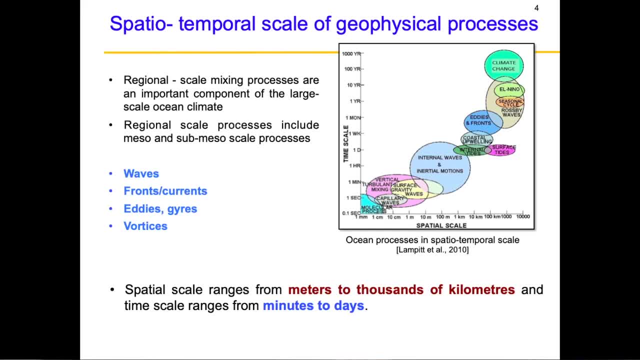 any places. so that is why weather is such a complex topic and one should understand and respect it. and whatever we are able to do with a limited topic- sorry, with our limited knowledge and with a limited modeling capabilities- should be appreciated. and of course we can do better as and when we understand. 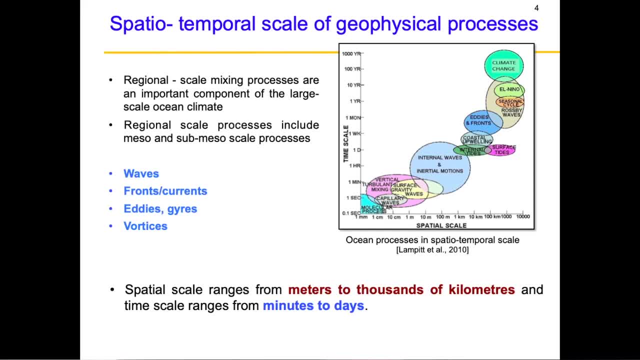 the processes in a better manner. and that's why the importance of dynamics plays a very important role, because unless you know, until you appreciate the dynamical aspects, then you cannot actually make any improvement in the weather arena. okay, so, as an enthusiast, it's important to appreciate and appreciate the dynamics. okay, so, as an enthusiast, it's. 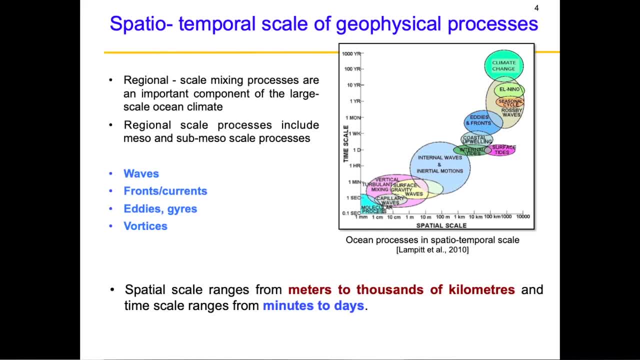 important to appreciate and appreciate the dynamics. okay, so, as an enthusiast, it's, you can follow models, but at the same time you understand what are, what is the which particular spatial feature actually caused that event, and then try to look more into that and try to refine that process and include that process in 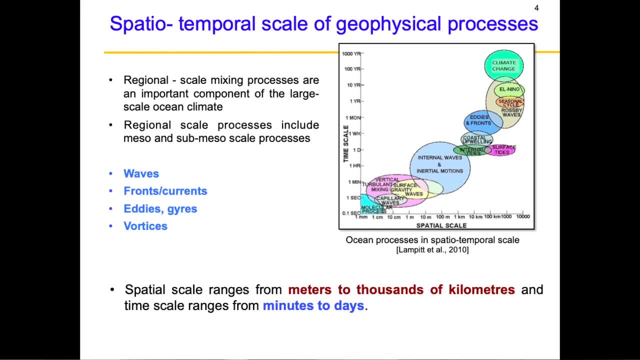 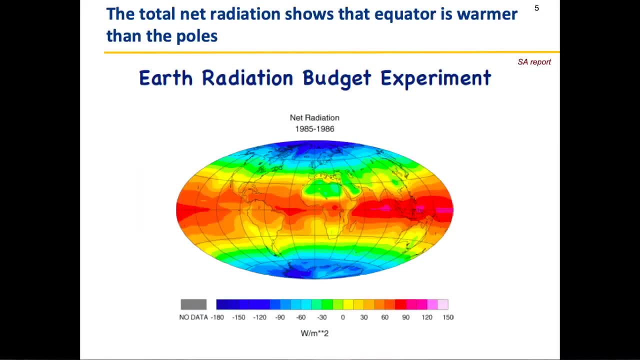 the model if it doesn't already exist, and that's how you improve your scientific frontier, and so you improve your weather prediction capability. all right, so now that move. enough about why weather is a complex system, but I have tried to explain in a much better manner why it is so, so I hope it keeps a. 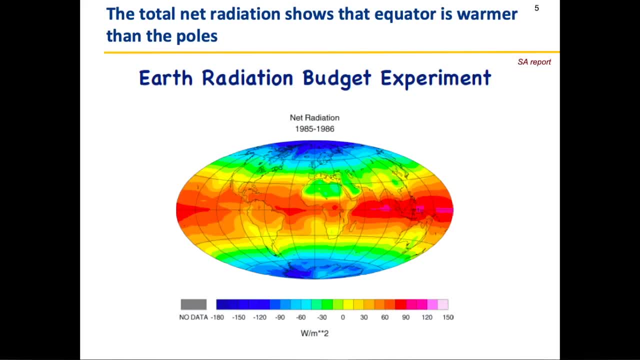 clear idea to you now. but now what happens in in terms of convection. so we know that earth in the. so if you look at the tropical region, equator, then it is hot, whereas polar region is cold. so that drives a convection and very important, without convection you cannot have these. without convection then air wouldn't. 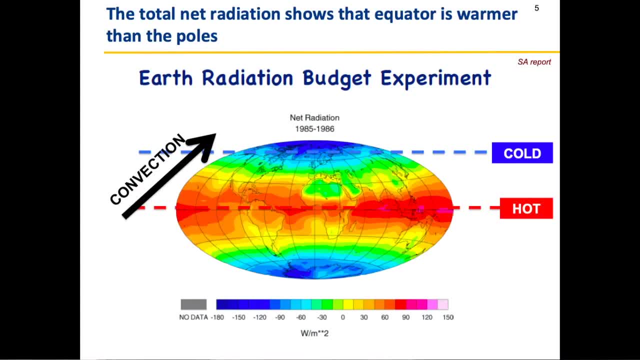 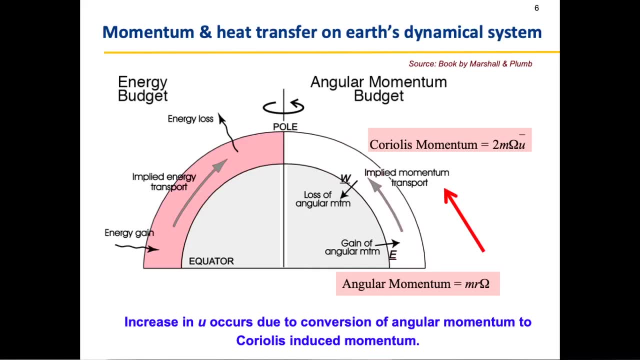 flow, it would be rest at rest. so this is what causes the restless air, which is the convection. the second thing that actually aids in the restlessness of the air is the momentum. anything that is moving has a velocity and anything that has a velocity and the mass will have automatically a momentum. so, if you are 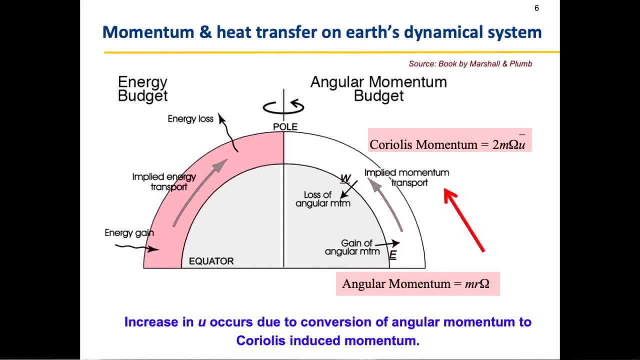 sitting, you don't have any momentum. as you, as you start stand up and start moving, you are a person with some mass and then if you start moving with velocity V, then you have actually gained a momentum and that's what pushes you forward or pushes you back. okay, that's exactly what happens with air also. it 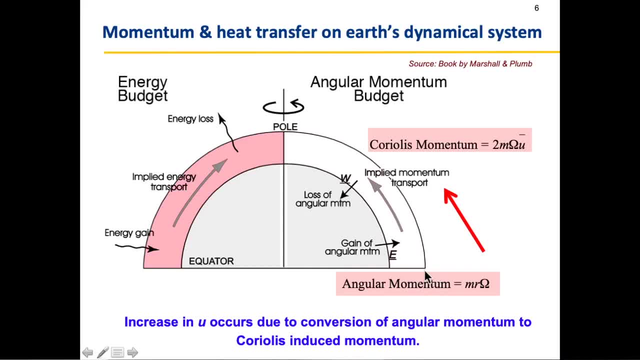 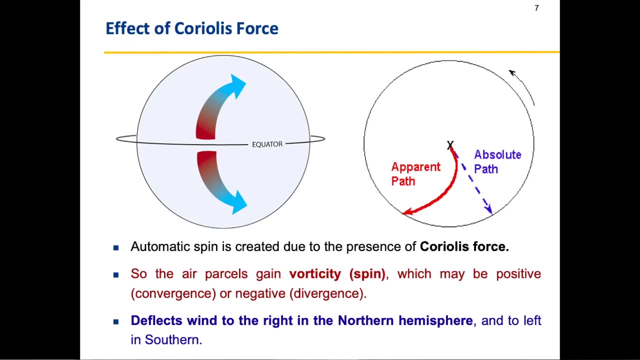 attains momentum and that particular momentum, the equator, it is angular momentum and as it moves meridionally up, it converts into Coriolis momentum, and that's how the effect of Coriolis also comes into picture. and the third thing is the Coriolis force itself, which is actually the rotation, due to the rotation of the 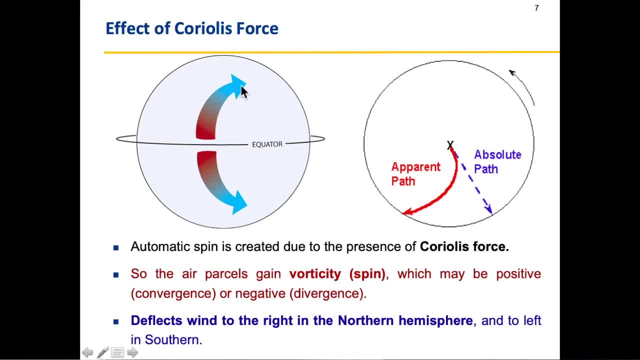 earth. if the air was not rotating, then any parcel will not get deflected. but thanks to the rotation presents, any parcel in the in the earth will get deflected to the right in the north-right, cioè the right in the north-right means to the left, which is L, and the L is the L is the. 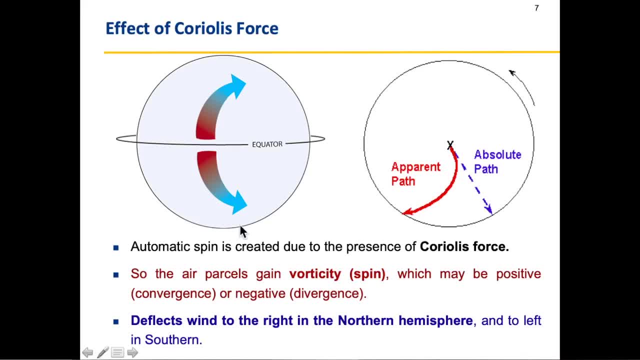 northern hemisphere and to the left in the southern hemisphere, and this automatically creates a spin and that's why parcels have automatically a tendency to gain vorticity in rotating frame of system like earth. and that's why vorticity is always a very important aspect, because vorticity is what causes the rotation and rotation is what causes convergence and 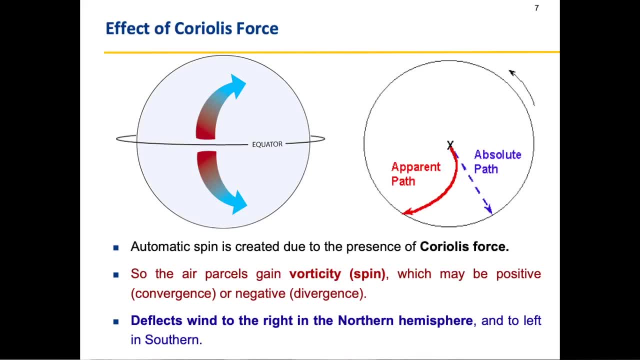 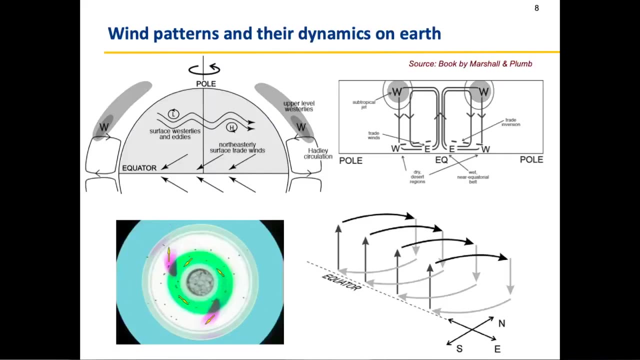 convergence is what causes the moisture to get updrafted, and as moisture is updrafted, then you automatically form clouds. okay, so this is where these three things- convection, momentum and Coriolis- is what governs the bigger aspects of weather. so, thanks to all these three things that 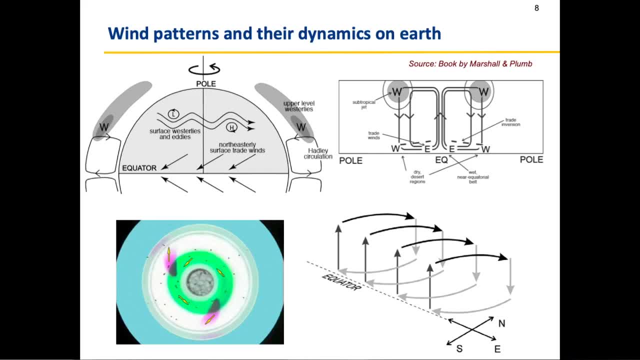 we just talked about the convection, the momentum and Coriolis. a system, a parcel near the equator will rise up because of the convection. it will move up because of the momentum that it has gained and then, because of Coriolis, it will be deflected to the right and then it will move down, and this 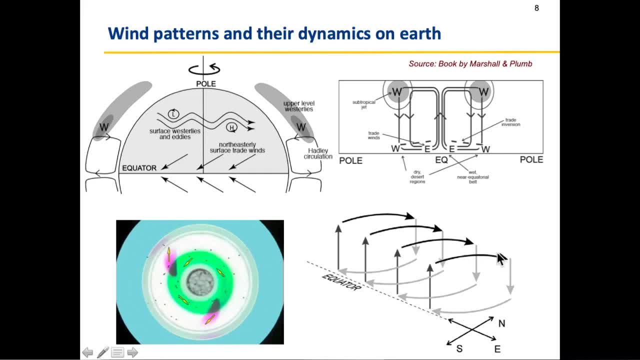 is what you call as a loop. okay, so that's how you actually attain the westerly winds, and then it will move down. and this is what you call as a loop. okay, so that's how you actually attain the westerly winds at the mid-latitude and easterly winds near the equatorial region. so 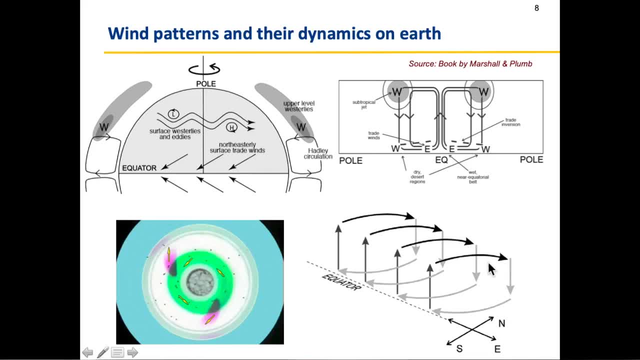 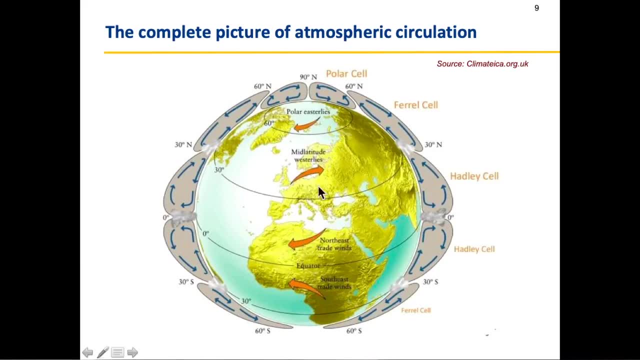 this is the Coriolis momentum and convection as the reason why you have these east-west kind of trade winds that occur. and the complete picture is this: where you have easterly winds near the equator and you have westerly winds at the mid-latitude and that actually causes the 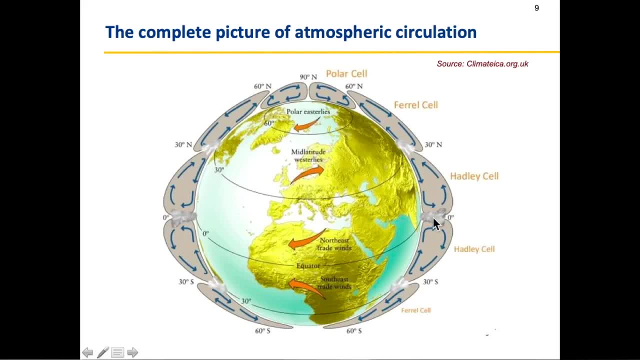 formation of a cell which is known as the Hadley cell. and that Hadley cell plays a very important role because it the you have Hadley cells, Hadley cell, in the northern hemisphere and the southern hemisphere, so the point where the two cells meet, that's where the winds also meet. 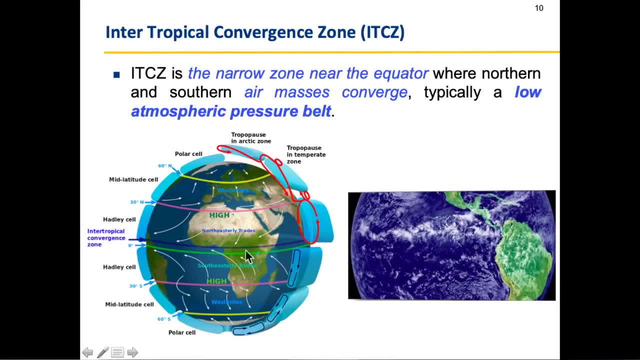 from the northern hemisphere and from the southern hemisphere the winds meet and wherever they meet they create a zone of strong convergence and a low pressure built, which is what we call as the inter-tropical convergence zone, ITCZ, and the ITCZ can be seen from any satellite image as a thick 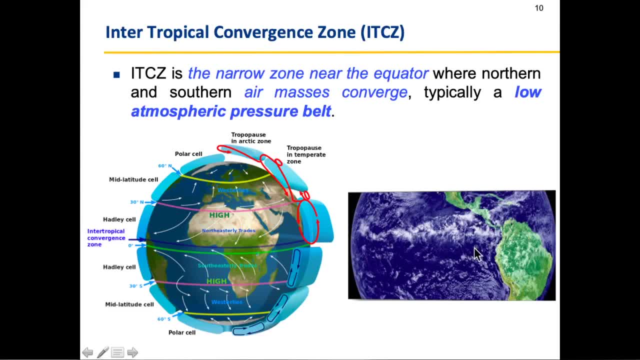 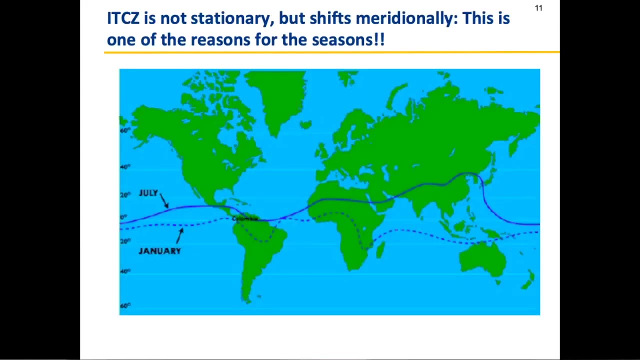 dense mass of thunder clouds which actually have the tendency to give a lot of rain. and the ITCZ is not stationary, it is moving. it moves meridionally, up and down, so it has a southward as well as a northward movement, and that actually is what gives you the monsoon season. so what happens is ITCZ is. 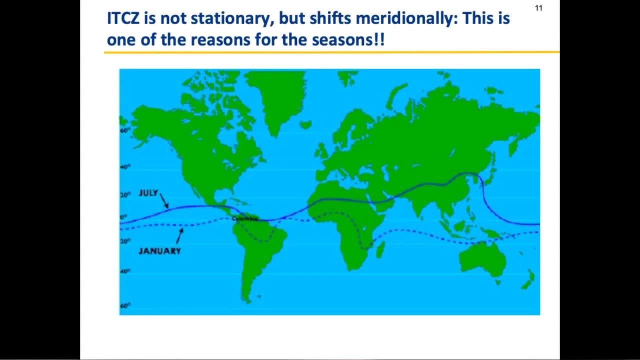 not stationary because. so again, ITCZ formation is very important. the basics is what I have explained. if you take out convection, if you take out momentum- you could take out Coriolis- you will not have Hadley cell formation. if you don't have Hadley cell formation, you will not have ITCZ. so 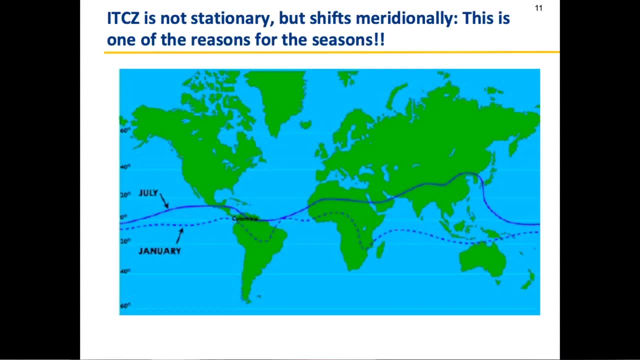 if you want to actually understand the ITCZ movement then you actually need to look into Hadley cell formation and then how the Hadley cell moves. and if you want to look at the Hadley cell in a more microscopic manner, then you need to understand convection momentum and Coriolis. so 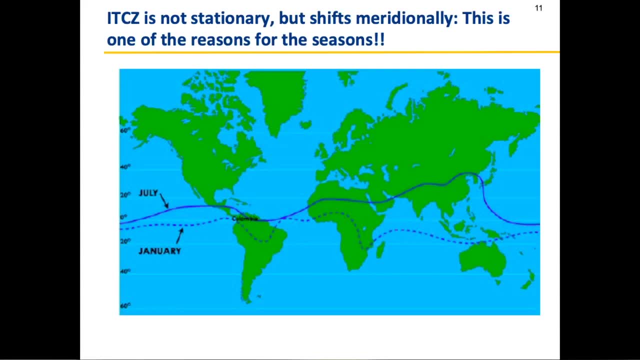 that's how basics are the building block of weather. okay, so that is what I am trying to do in this video, or lecture, if you may. so ITCZ actually moves up and down. as you can see, during January it is very close to the equator and as you transition to the month of monsoon, 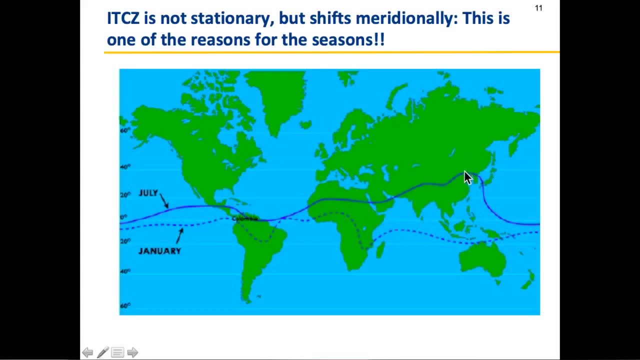 for India, then you see that ITCZ moves up. so this is now. the Hadley cell has been pushed up north. the northern part of Hadley cell is now here, the southern part of Hadley cell is here and wherever they meet, that's where you have ITCZ, which is a tropical convergent zone, and this is 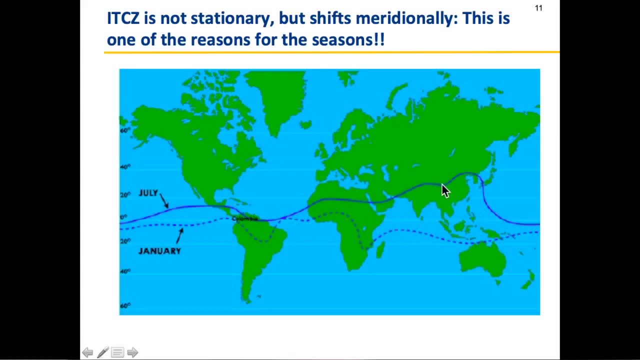 the belt of low pressure, so strong low pressure exists near the Himalayan subcontinent and that is what pulls the trade winds from Africa towards India and that's what gives you this Somali jet, about which I will talk later. but this movement of ITCZ is very, very crucial for monsoon, as it 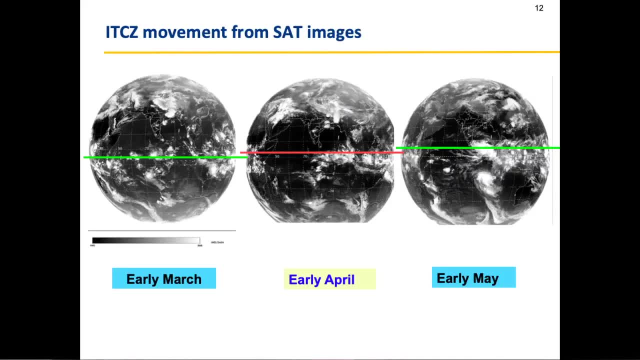 is the northeast monsoon, so this movement of ITCZ is very clear during March, April. you can actually look at the satellite images and you can clearly pin down where it is moving. and again, like I said, the ITCZ zone is the very thick, dense cloud, thunder, thunderstorm cloud, so you can 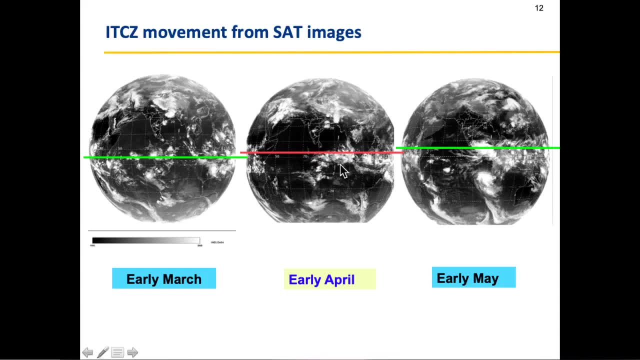 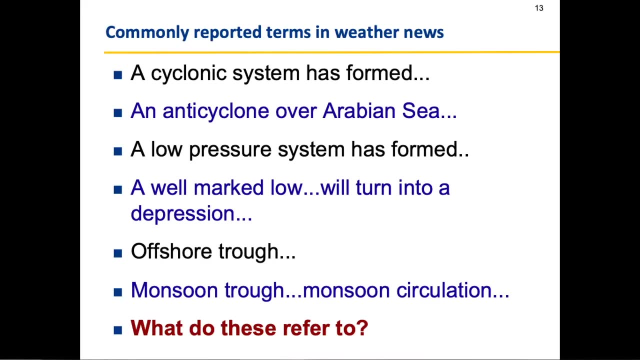 actually figure out where the ITCZ is lying just by looking at the cloudiness quotient. all right, now we understand what is the bigger scale synoptic system, like the Hadley cell which aids in the monsoon formation, and all those things. now let us look into some specific terms. 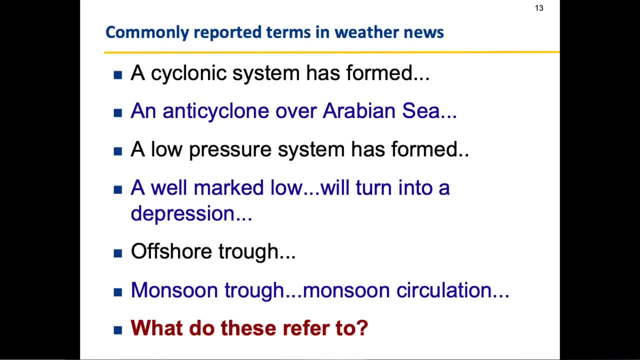 where we commonly hear these terms in the weather news, which is: a cyclonic system has formed, an anti-cyclone exists over Arabian Sea. a low pressure system has formed, a well marked low has formed which will turn into a depression. an offshore trough has formed, a monsoon trough, monsoon circulation. so 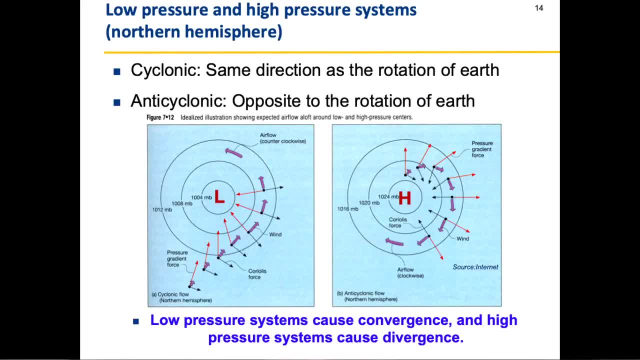 many terms. so what are what do these refer to? okay, so a cyclonic system is nothing but a system which is rotating in the same direction, the rotation of the earth. okay, so in the northern hemisphere, if the system is rotating in a anti-clockwise direction, so if the winds are in the anti-clockwise direction, then you have 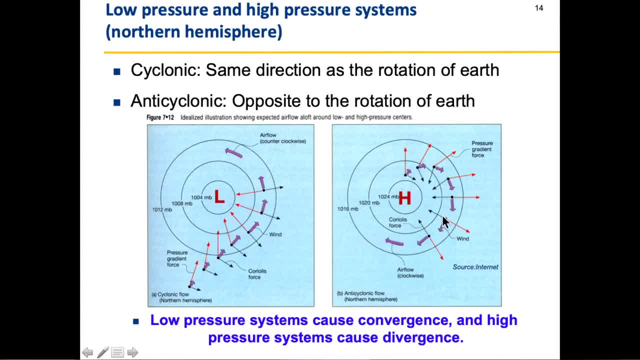 something known as a cyclonic system, whereas if the winds are in, the winds are clockwise, then you have something less an anti-cyclonic system. okay so, and this is actually this: movement of this winds is what causes the low pressure and high pressure systems so effectively when the 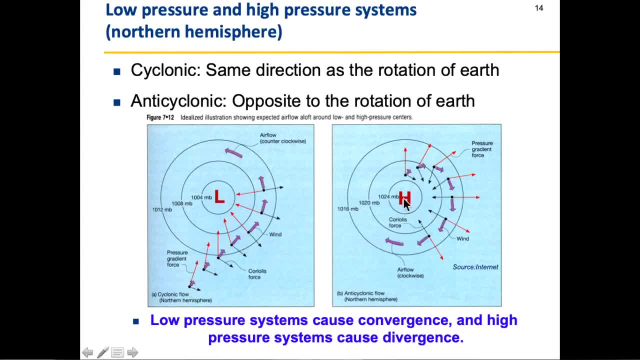 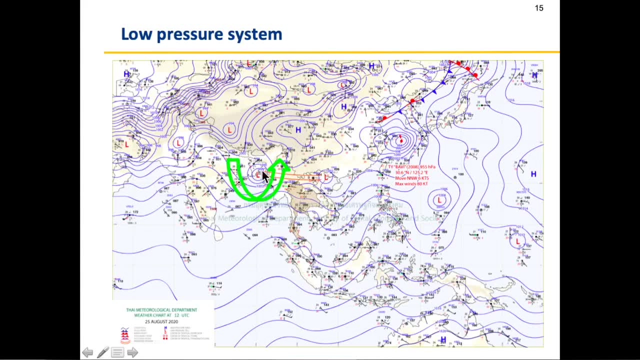 winds are cyclonic, then you have low pressure, and winds are anti-cyclonic, you have high pressure. okay, so you can actually find out these lower pressure and high pressure systems by looking at the pressure charts or wind charts. so this is a low pressure and if you look at the wind chart, then 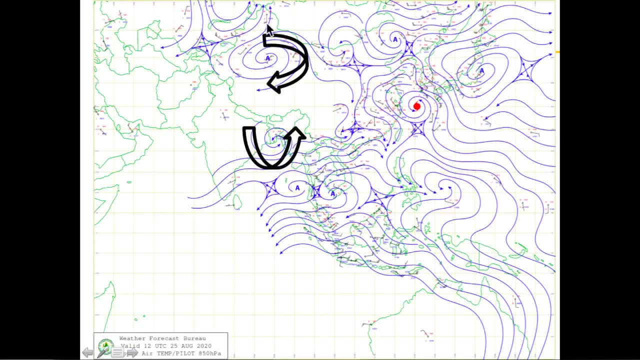 it's a low pressure because the winds are cyclonic and winds are anti-cyclonic, which means winds are clockwise in the northern hemisphere. so that is what is the anti-cyclonic or high pressure zone. okay, so cyclonic and anti-cyclonic are basically the broad, broad terms. 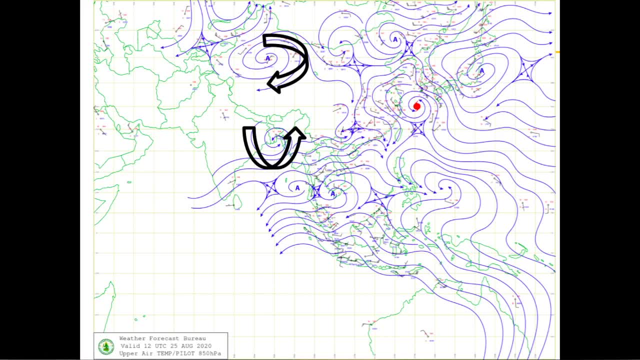 so, like any, any movement of wind, either clockwise or anti-clockwise, is termed as anti-cyclonic or cyclonic. so if the winds are moving counterclockwise, then it is a cyclonic pattern, the winds are moving clockwise and this anti-cyclonic pattern, then you have 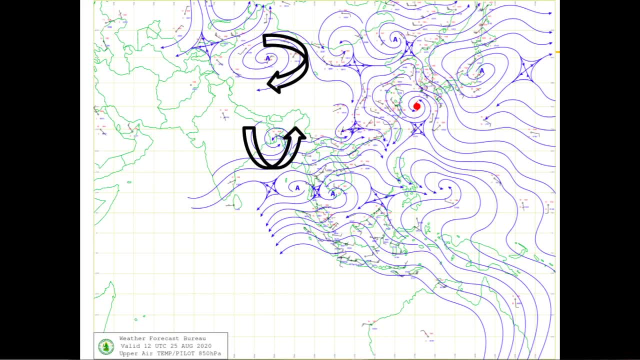 the next step, which is low pressure. and high pressure, uh, that actually comes into picture when the pressure drops, uh drastically to a value at the center. so now the system which is forming gets a little bit more organized. okay, so winds can actually be very disorganized, in the sense that they can. 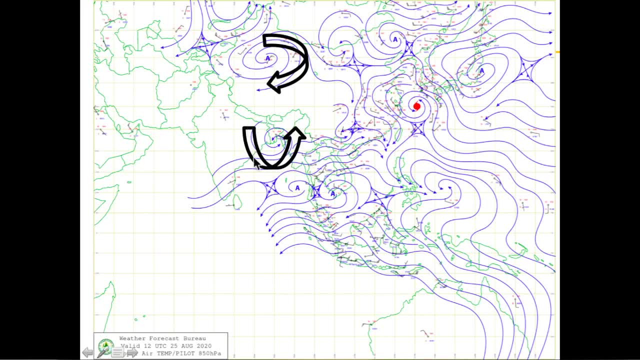 they would not kind of form this loop. but as they try to form this loop, then you actually call them a low pressure or high pressure systems. okay, uh, whereas if the winds so this, this is not an organized system, but this is still a anti-cyclonic wind, so it is a anti-anticyclonic. 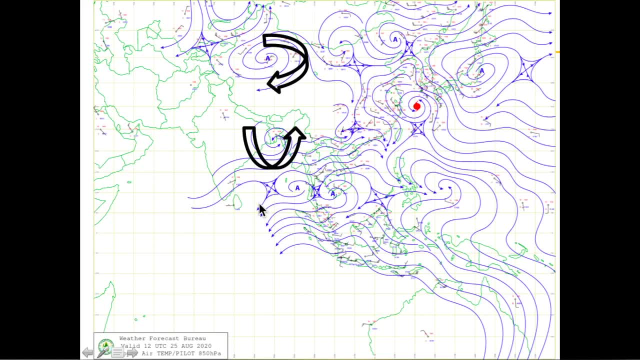 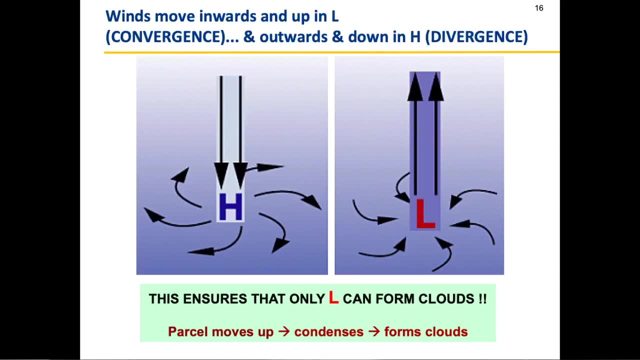 motion, because the winds are moving in the clockwise direction. okay, when the winds actually become more organized, then only you give them the name, such as low pressure, and when they become even more organized, then you get into depression, depression. and when they are fully organized and have an eye, that's when you call them the cyclone. uh, so why is this important? the movement of the 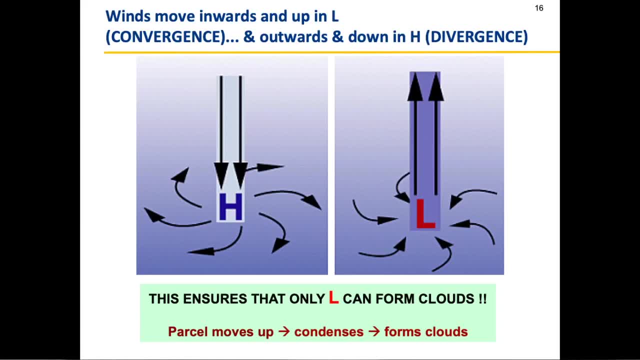 winds. that's what gives you convergence and divergence. so when wind masses converge, then they actually is a low pressure system, so where the air masses move in and they move up, they bring moisture and they lead to formation of clouds, whereas high pressure systems they allow winds to come from top to bottom, so that's why cloud formation is not possible. so high pressure- 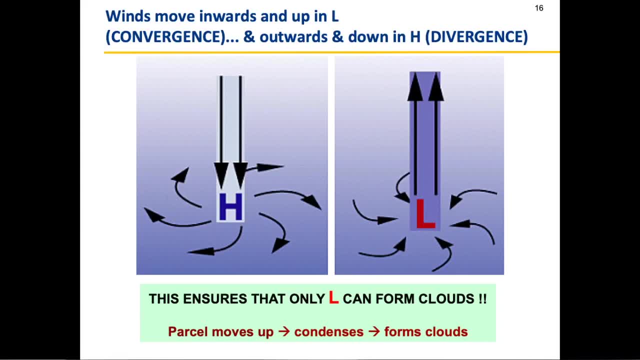 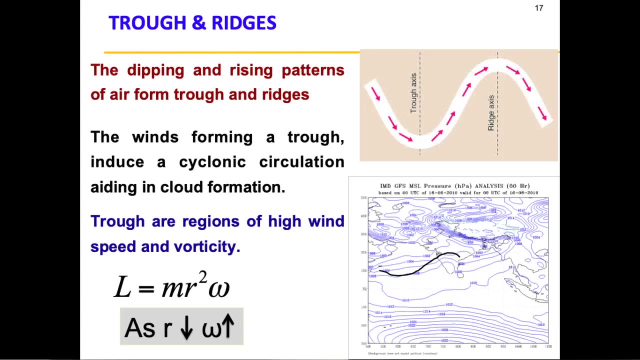 is always associated with clear skies, whereas low pressure is always associated with cloudy sky, which is going to give you rain probably. then you have something known as trough and ridges. trough and ridges are again wind patterns. everything is related to wind here- wind patterns which are not actually forming a closed loop, but they are going up and down. so this is a trough. 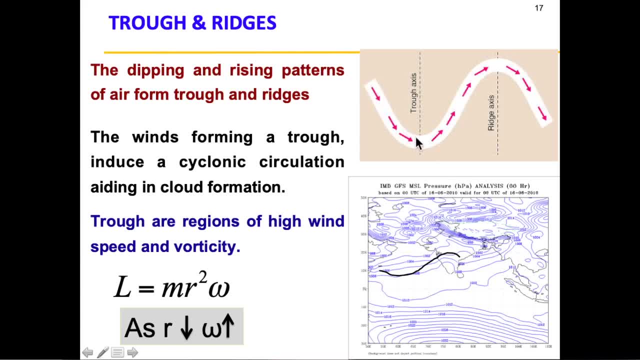 this is a ridge, okay, as the wind is moving from west to east. this is a trough. this is a ridge because wind has dipped down whereas wind has moved up. so all you have to do is you have to other way to enter, a other way to talk about trough and ridges, not the dip and upward pattern. 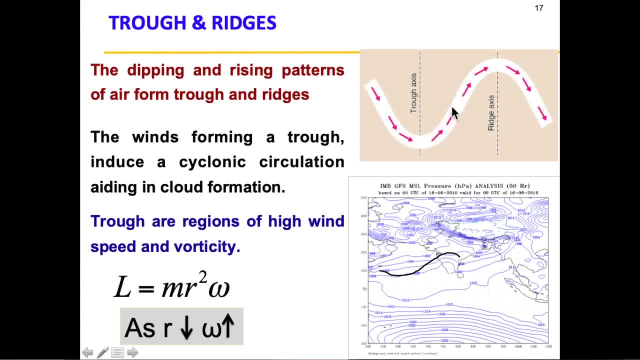 but what kind of movement, what kind of pattern they are making. so this wind is making a cyclonic pattern. right, because as this wind is moving, if i close this loop, hypothetically speaking, then i will have a anti cyclonic system, because winds are anti-clockwise, whereas when this is moving here, 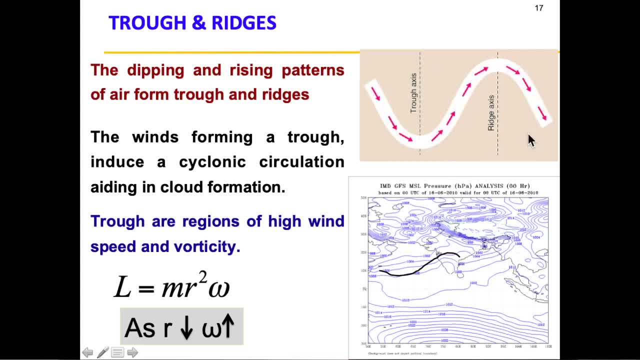 if i close the loop, then it is a clockwise motion. so anti-cyclonic winds. so the movement of cyclonic and anti-cyclonic winds which don't form a loop is what is called as trough and ridges. so trough is a cyclonic movement of wind which has the potential to deposit vorticity. okay, because it. 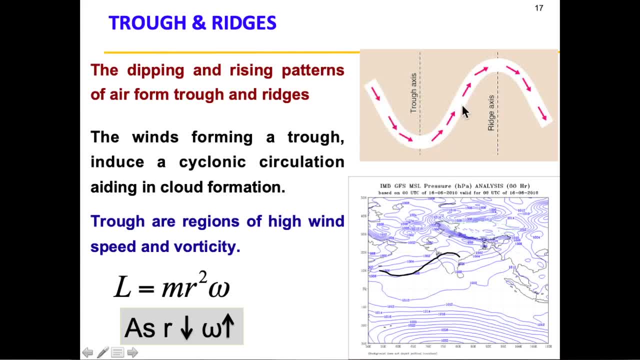 is moving in the cyclonic direction and that vorticity is the reason why convergence will happen and it will lead to formation of clubs. and the other very important thing about trough and ridges is that as the radius of curvature of the trough keeps reducing, then from the 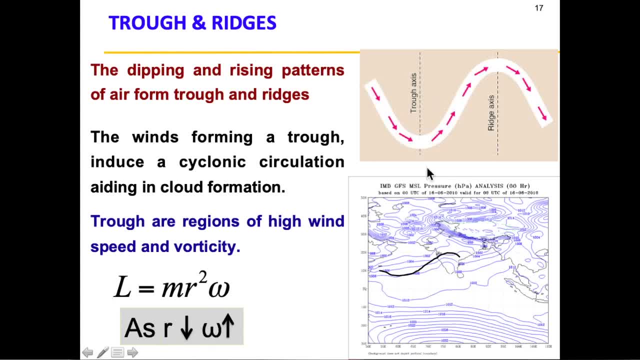 conservation of angular momentum. you can see that as radius reduces the radius of what i'm talking about, if this becomes more sharper, so the peak is more sharper. so you can have two things: you can either have a very long trough or you can have a very sharp trough. so sharp trough are dangerous because they will lead to very strong winds. 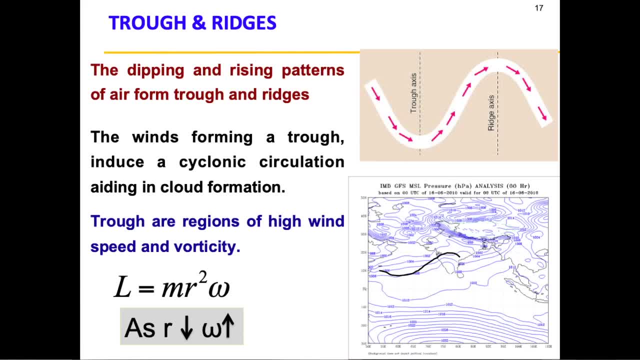 and strong winds means high vorticity, and high vorticity means more convergence and more dense clouds formation. this pattern of trough is what is very important for offshore trough is what we call, during monsoons, the southwest monsoon system, and that is what gives. 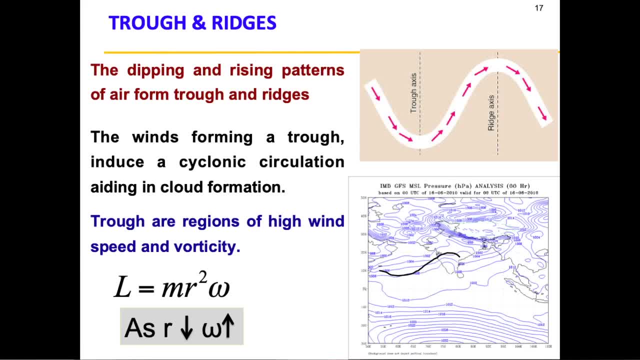 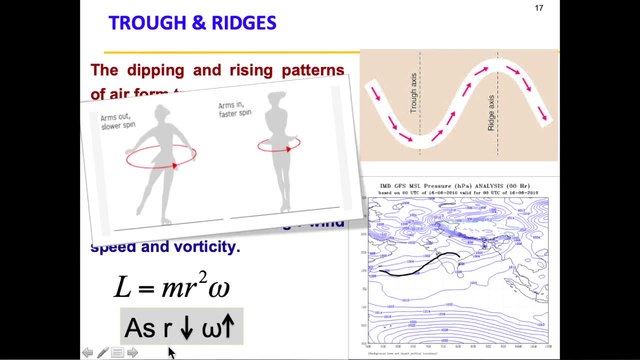 the wind to the west coast of india. i'll explain that probably in the next slides. so this is basically why systems which are more, which have r reduced when r reduces, why you gain angular momentum, is from this classical physics laws, where ice skater spins faster when she brings. 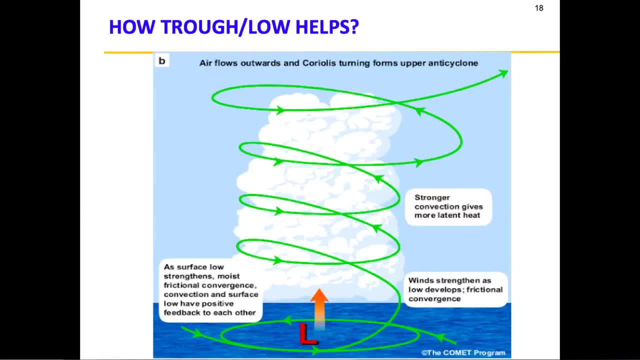 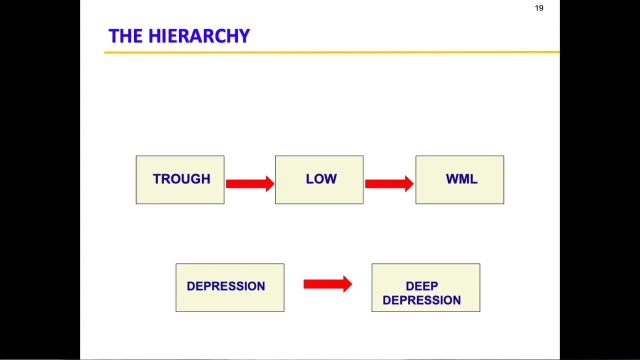 her arms in. so how trough and low helps. they create a situation where convergence can happen. high vorticity deposition- and uh, they will. strong winds will bring in a lot of moisture and they will eat up trough, forming clouds. so what is the hierarchy? the first thing is trough, because you don't have any organized pattern. so 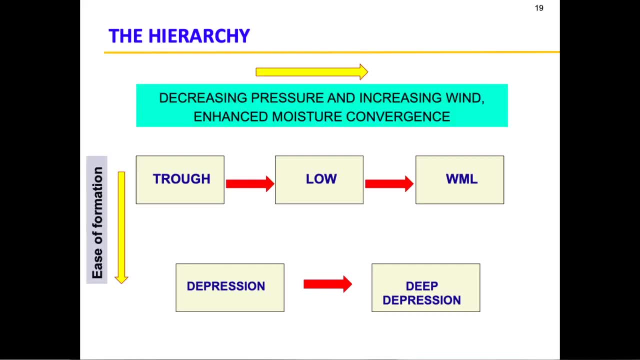 winds moving, cyclonic, uh, form a trough, and then you have low, and then well marked low, as things start organizing so and you have a distinct pressure present at the center. then you have a low pressure. then, as the pressure keeps dropping, you have the well marked low, the 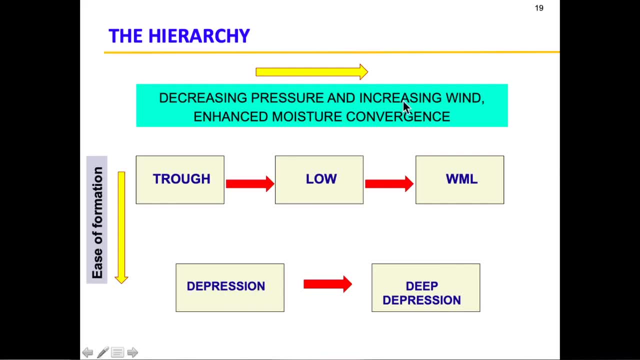 depression, deep depression and then cyclone. so the difference is decreasing pressure and increasing. this has less, says the. as you keep going, the pressure drops and winds also increase and enhance moisture convergence- convergence ease of formation trough is the easiest to form because you don't need a very organized system, you just need dipping and dipping pattern of. 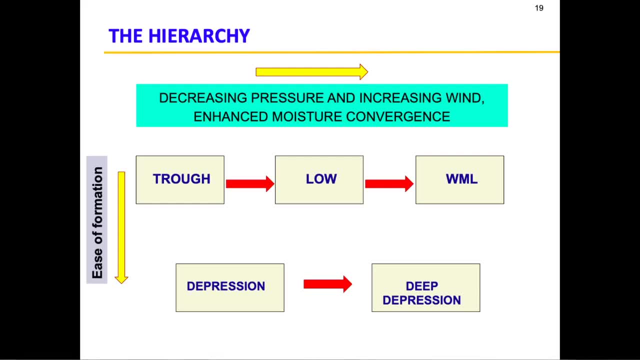 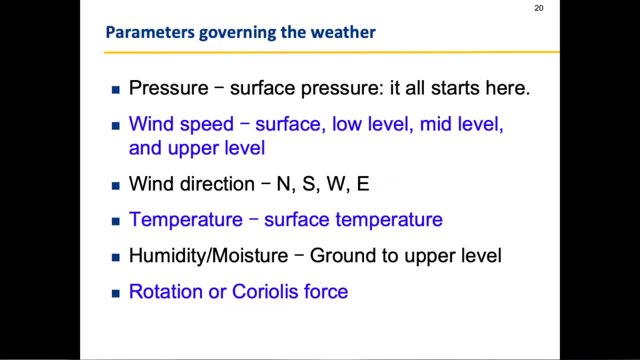 winds or cyclonic pattern of winds. so that is easy to form. as you keep going, deep depressions are difficult to form. pressure again governs the system. so pressure, winds, temperature, moisture rotation, these are the things that govern the weather. this we have already talked. i just spoke. 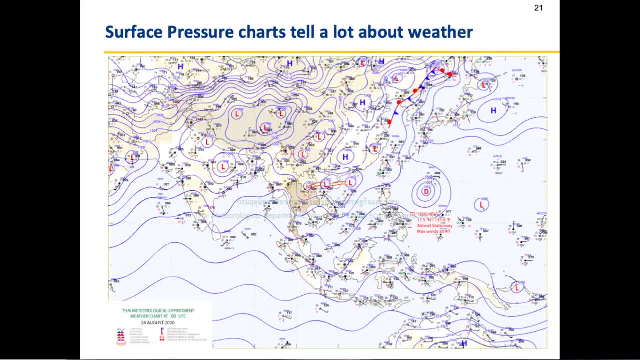 about all of these and you can actually learn a lot from pressure charts. if you look at a simple pressure chart, you can actually see where are the low pressures and you actually on the are on the lookout for the low pressure systems because, that is, those are dangerous and this is typical monsoon. 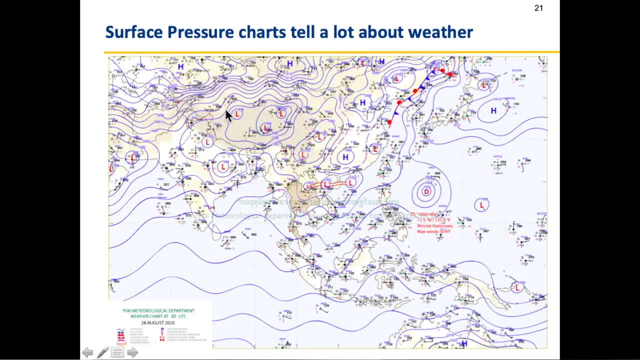 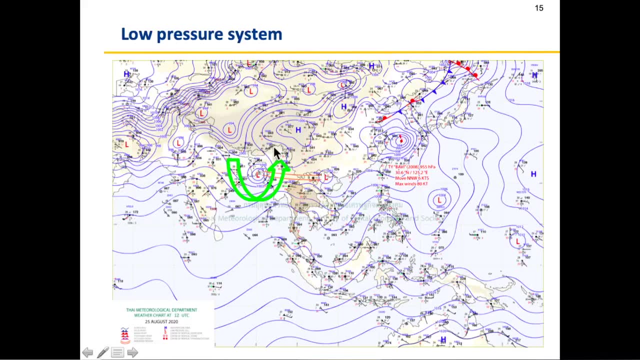 season- i think this is in august- you see a lot of low pressure uh in this region. this which is where the itc z has moved, because in july, if you remember, i showed uh the itc z has moved in july z location. see, it's near foothills of himalayas and that's where a strong low pressure exists. 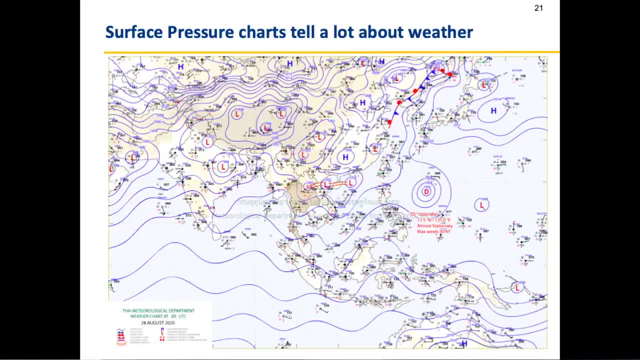 and that low pressure pulls in a lot of winds and moisture and that's how you get- and this is a trough. you can see a dipping pattern, cyclonic pattern, this is a trough, and that trough gives a lot of rain to west coast of india. so you're on lookout for these kind of systems. 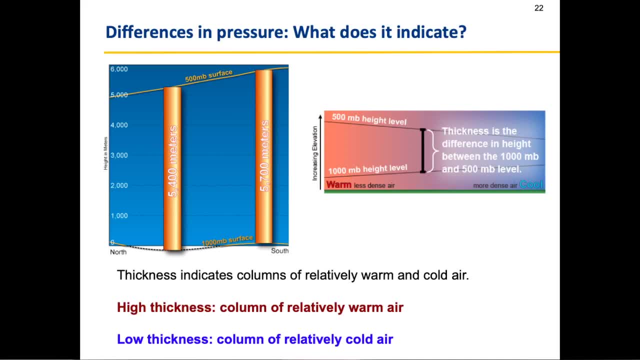 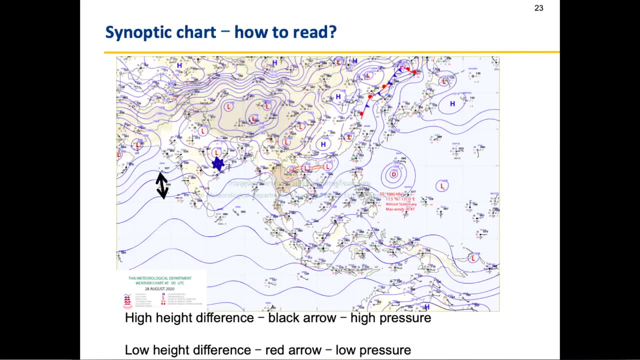 from pressure charts. uh, what does pressure actually mean? so, in very simple terms: high thickness. if the lines are far apart, then it's high pressure. lines are near, they are low pressure. so you can again clearly see this is a high pressure because lines are far away and as the 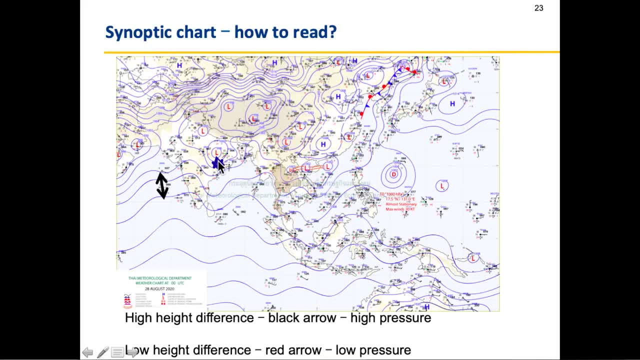 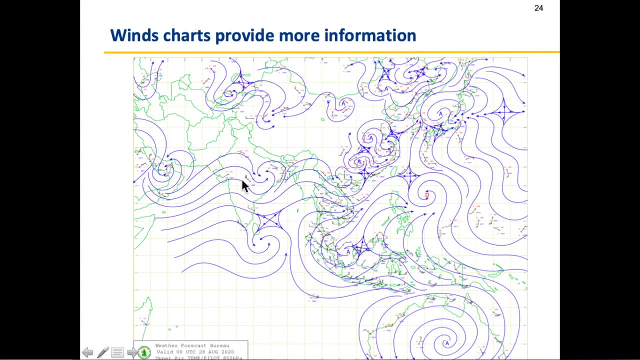 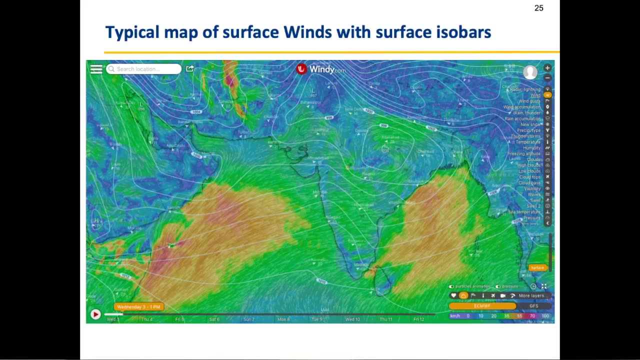 lines become closer and closer. it's a high pressure. okay, winds provide very good information. i've already already talked about this cyclonic and anti-cyclonic winds, so i'm not going to dwell more. uh, typical, what you actually do is you put both winds and isobars, or pressure, on the same. 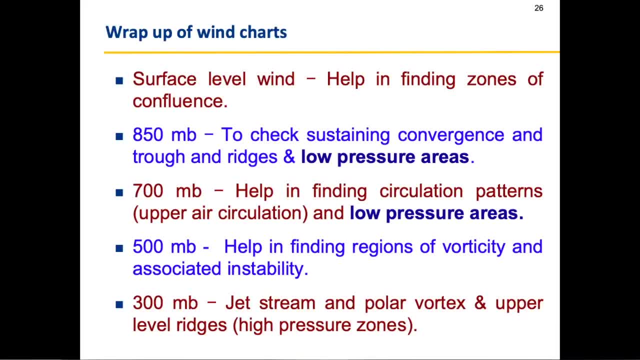 chart and you get a lot of information. okay, just a wrap-up of wind charts and pressure charts. so so, surface level wind help in finding zones of confluence, which is where the winds are meeting and where the updraft will happen. 850 mb pressure charts actually help in checking the sustenance. 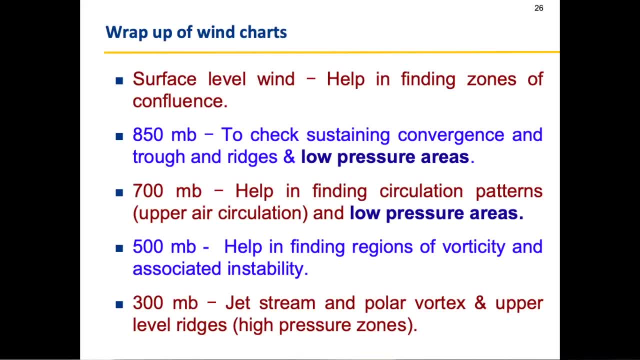 of convergence, whether the convergence will go to higher levels and whether it will result in a form, excuse me, result in the formation of low pressure or a trough and ridge of kind of a pattern. then 700 ml bar level is helpful in finding circulation patterns which are either: 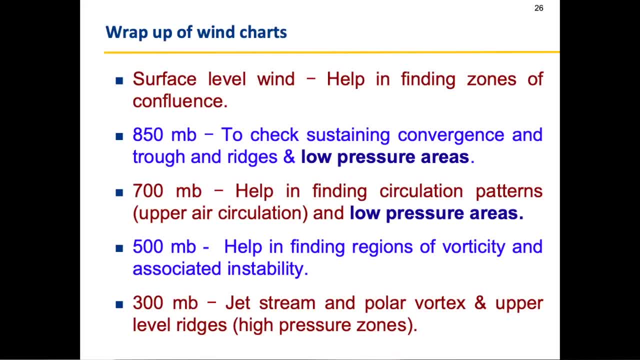 low level circulation or upper level circulation and also low pressure areas. millibar is very, very important because it will help in finding the regions of vorticity and associated instability. so if you are interested in finding deposition of vorticity, then a 500 millibar level is the most important to check. 300 millibar is very important during winter time. 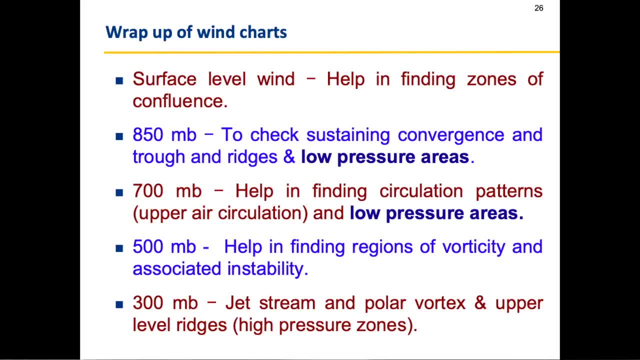 where you actually look for jet stream and polar vortex kind of systems and when a cyclone has formed, you actually look at the 300 millibar level for upper level ridges, or ridges are high pressure zones. so because the cyclone tends to take the move along the the ridges, 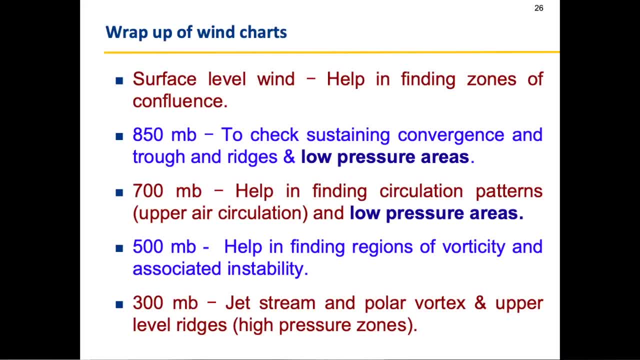 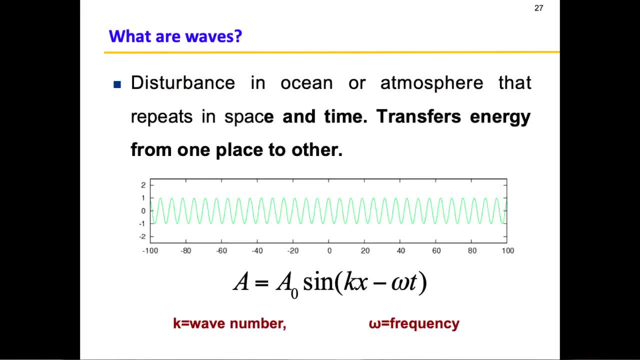 so these are the importance of the wind charts at different levels. and again, when i say wind, i don't only look at wind, i also look at pressure, because those two go hand in hand. the next important aspect, when you talk about weather, is waves, because the waves is the one that actually 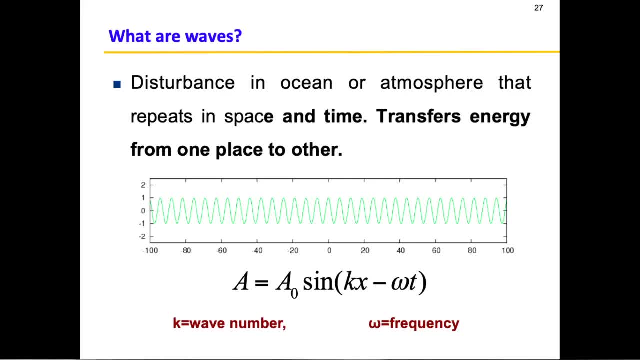 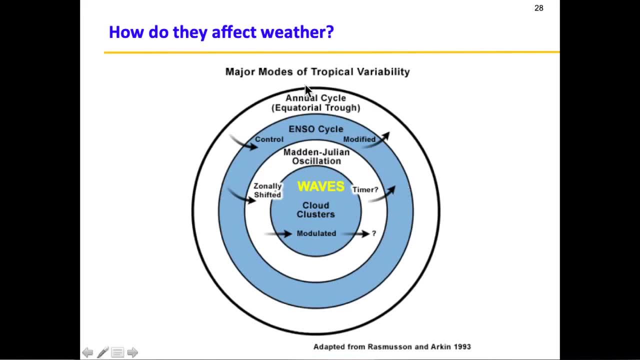 carry energy from one place to the other and they transfer energy from one place to the other, resulting in a lot of energy transfer. how they affect is that you have major modes of variability- long leno, it's a very long scale variability. then you have the manager in oscillation. 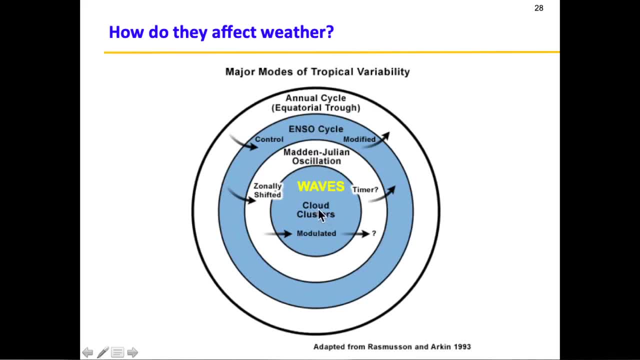 and all of these actually result in formation of clouds. but they result in formation of clouds through a very important mechanism which is waves, which are the which is like the middleman. so if you take out waves, then their interaction will not be there. so the the connecting point between any 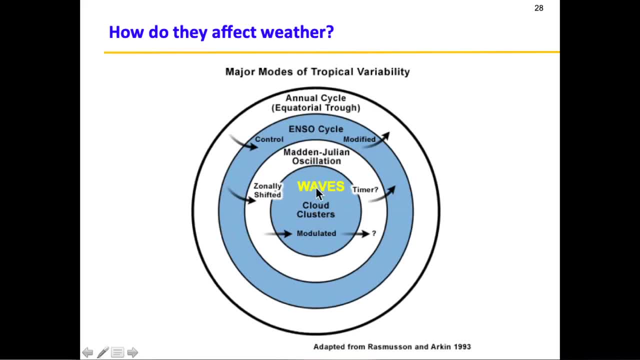 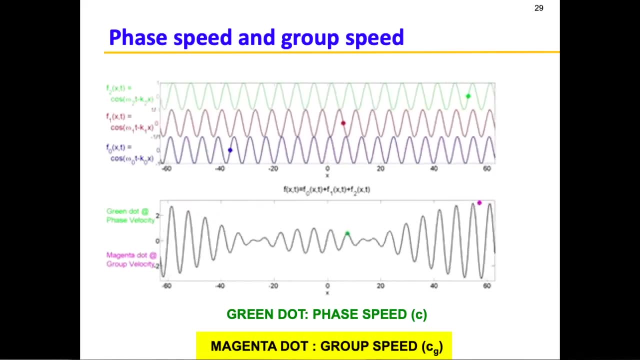 of these big structures and cloud is the waves. because they have to transfer energy, the waves come in many different uh can be characterized as dispersive or non-dispersive uh. dispersive is basically you have when you talk about waves, you have phase speed and a group. 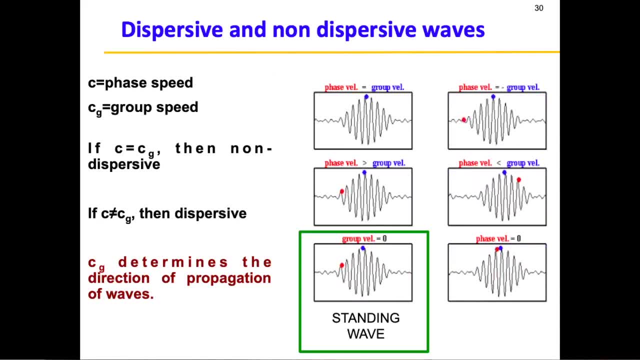 speed. phase speed is. phase speed is just the velocity at which the wave is moving. group speed is the transfer of energy. okay, so if the wave is moving and the group velocity and the phase velocity are the same, then what it means is that it means is that energy is transferred in the same. 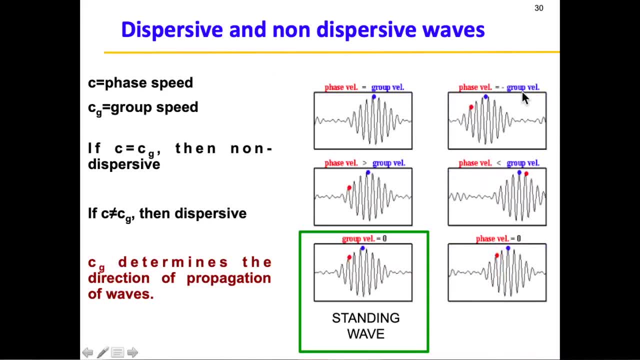 direction as the wave. however, if the phase velocity is negative, of group velocity, then you see the wave is moving in one direction, whereas the energy will move in the other direction. so blue and see, blue is the energy transfer. so, although the wave is moving in, uh, from left to. 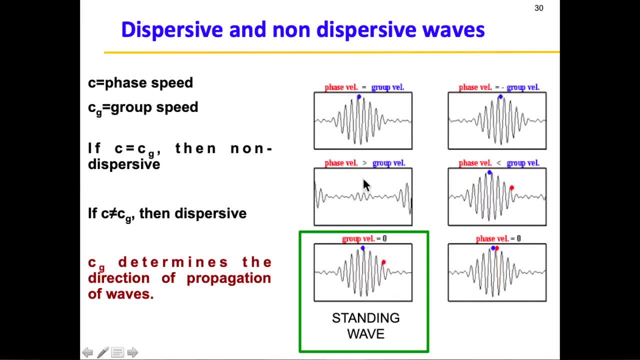 right, energy is being transferred from right to left, uh, and you can have other different aspects. so a dispersive wave is when, when the phase velocity and group velocity are not the same. this is a, this is a sorry, this is a non-dispersive wave. when both are same, then it is non-dispersed. 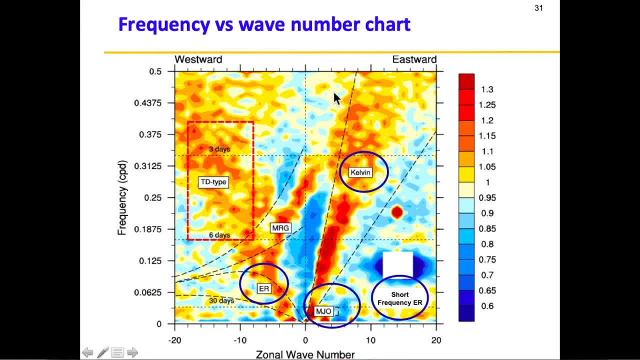 so you have different types of waves which are, uh, moving from west to east or east to west, and that alone is not important because, like i said, if they are dispersive, so even though, even though a rosby wave moves from east to west, but its energy will be always to the back of it, like it will. 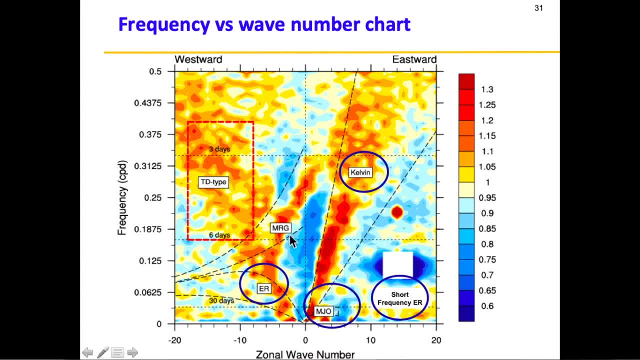 always give energy in the eastward direction because they are dispersive waves- uh, rosby, equatorial rosby wave or mrg wave. so even though their direction of movement will be from east to west, but the energy transfer will happen in the other direction. that's why it's very important. 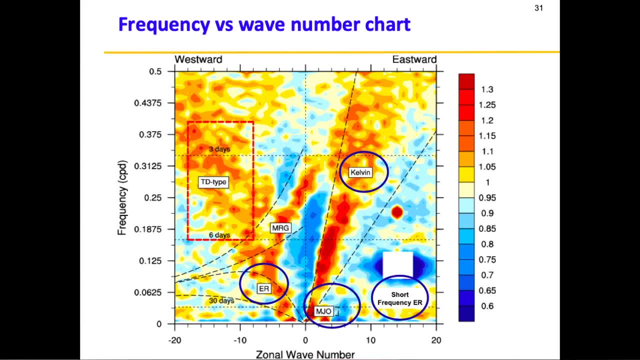 to understand these waves patterns and how they transfer energy, because otherwise you will actually get everything wrong in terms of weather dynamics. okay, so you can put a map and you can see. kelvin wave is a non-dispersive wave. kelvin wave is something which moves from east to west to east. they are always moving from west to east and they're 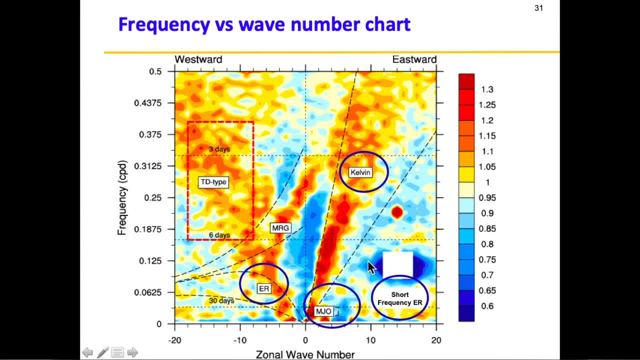 non-dispersive, that means they will transfer energy also in that same direction. and then you have mgo, which is uh, which is again a east to west wave, and it is again. it is again a non-dispersive kind of a wave, so energy will always again be transferred in the same direction. 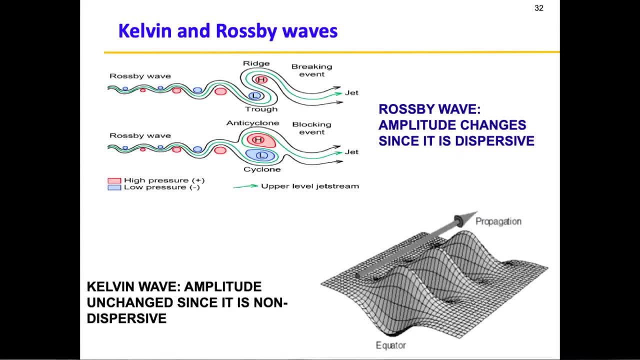 as the wave is moving. i can talk about two important waves, which are kelvin and rosby waves. it's not uh dispersive, so you see the amplitude has not changed. okay, so energy transfer will happen in the same direction, whereas rosby waves are very tricky because they start with small. 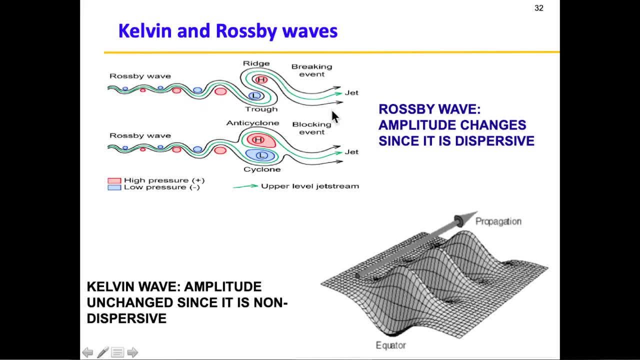 waves and then they actually gain amplitude and that actually results in a lot of trickiness. that leads to a lot of tricky feature because as the amplitude increases they can break down and they can transfer energy in a very random manner. that's why. that's why rosby waves are. 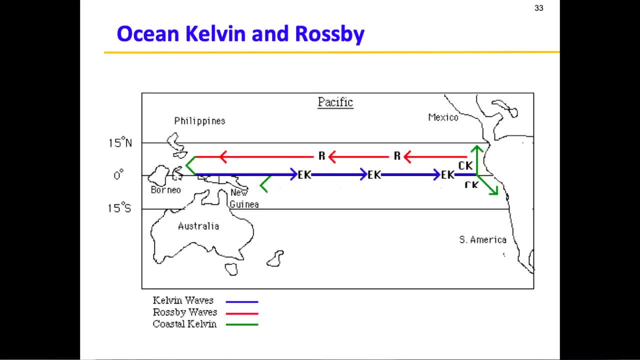 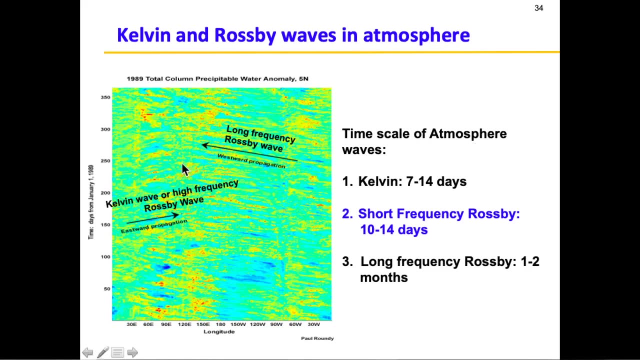 very tricky. um, you won't skip this slide not needed. uh, you can look for these rosby and kevin wave signatures through the movement. uh, whether the propagation, so the best propagation means raspberry propagation, means kilbin wave, and also the frequency, so rosby waves have a very high frequency, of 10 to 14 days, whereas kilbin waves are slightly shorter. 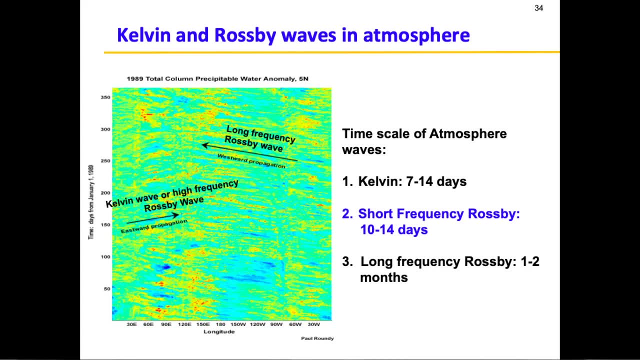 7 to 14 days, a long way free. there are also long frequency raspy wave which happen during monsoon seasons. those have a lifespan of one to two months, so they can linger around or move as a pattern of wave for almost one month or two months and these usually long, very long. 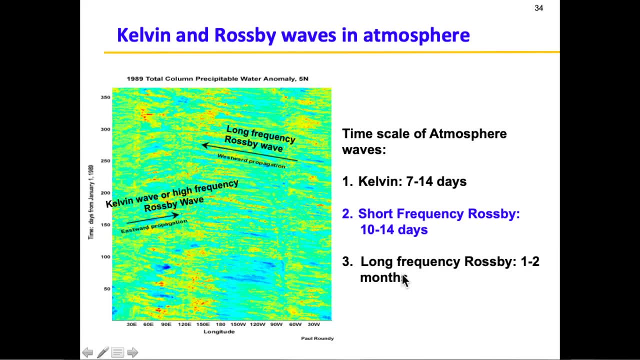 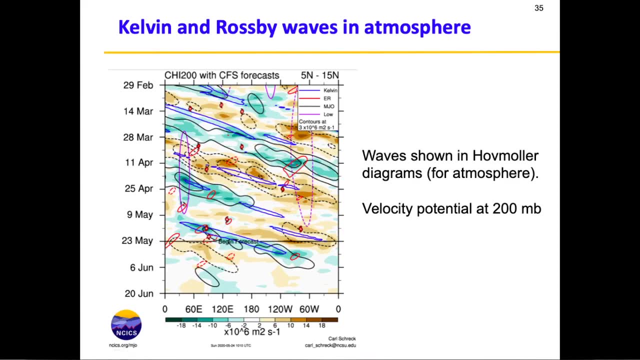 frequency rosby waves are seen in uh ocean, in the ocean, okay the atmosphere, you should usually have a very short frequency rosby waves. you can also draw, see the, the waves from the homoval diagram, which is the diagram of longitude versus the, versus the time and different waves propagation. 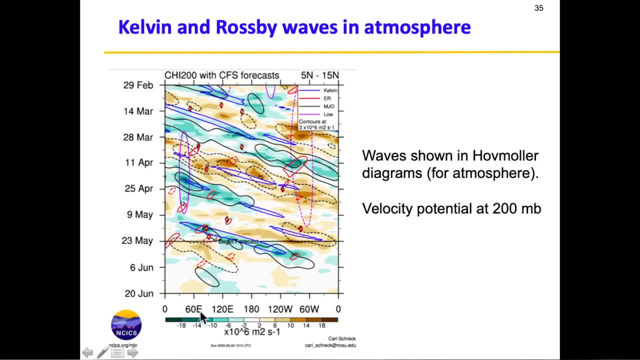 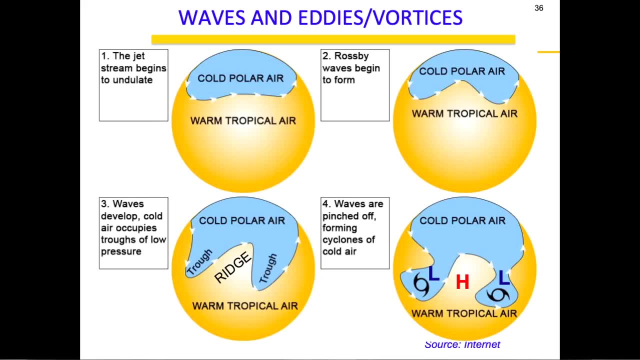 so you can find when that wave reached the which part of the continent, whether it was an indian ocean or the pacific ocean and those kind of things. and then you have the these waves, eddies and vortices. so, like i said, anything which is a mass of air. 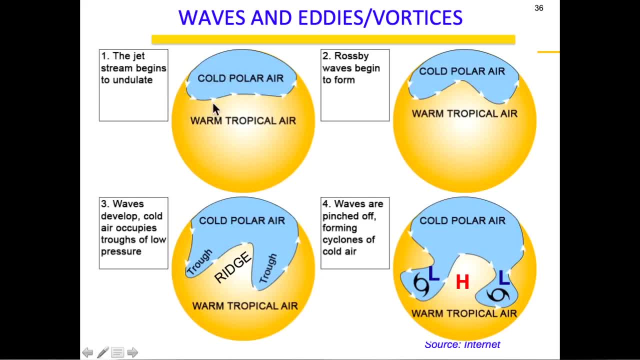 as these waves starts to. so take rosby: wave, the waves, this same picture. the wave started very small and then it went amplified, right. so same thing happens. so the wave started like a very small, high, frequent, high wavelength wave and then it started undulating. and then, as it undulated it, 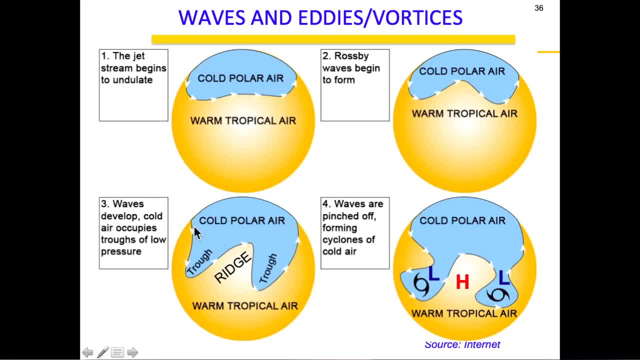 started splitting. as it split, it became a trough and a ridge, which means a cyclonic and anticyclonic system. cyclonic system then pinched off as a lower low pressure and the anti-circling system stayed as a high pressure. and this low pressure moves down, so that this is how the cold polar 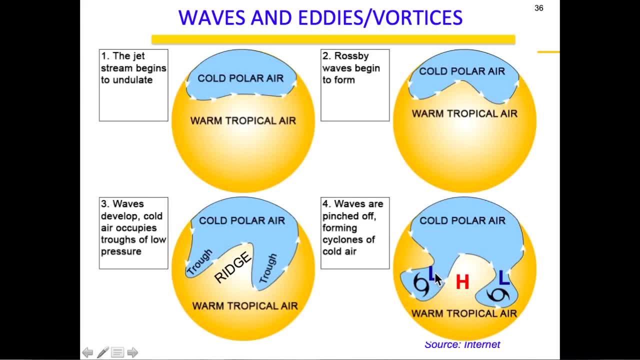 air during winter time is dropped to lower latitudes, and that is known as the meandering of jet streams, and that is how you actually have either systems forming, extra tropical systems forming like western disturbances, or you have in atmosphere i'm talking about. cyclones are different because they require ocean as well. this is purely in atmosphere, so or you have these polar 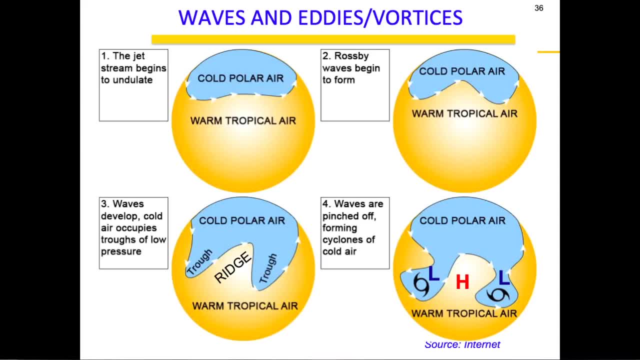 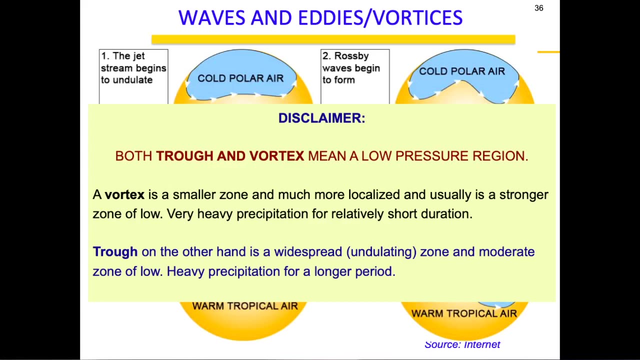 ices that drop down and come down to low latitudes, giving a lot of snowstorm, like extreme snowstorms. so the pinching of vortices are very common and this is where i want to put a disclaimer that both vortex and trough mean a low pressure region, but a vortex is a much, much smaller zone compared. 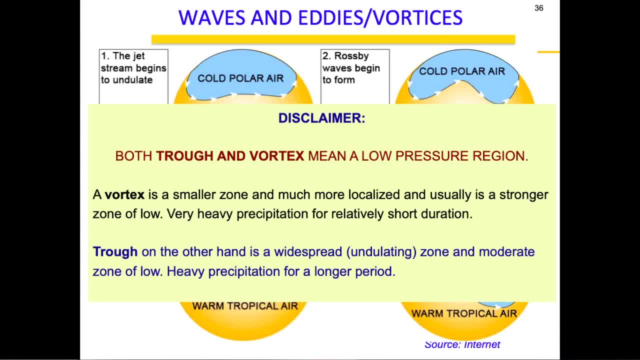 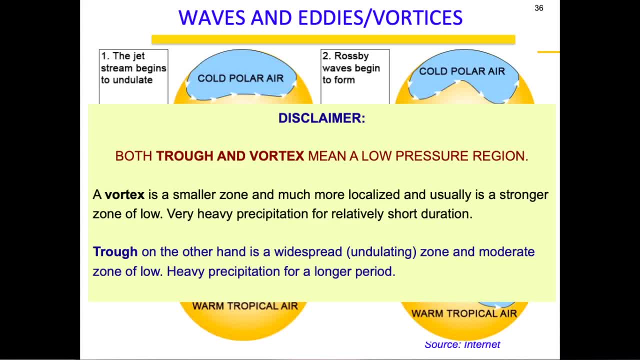 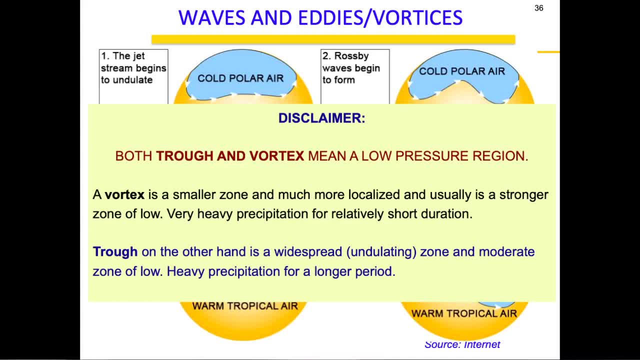 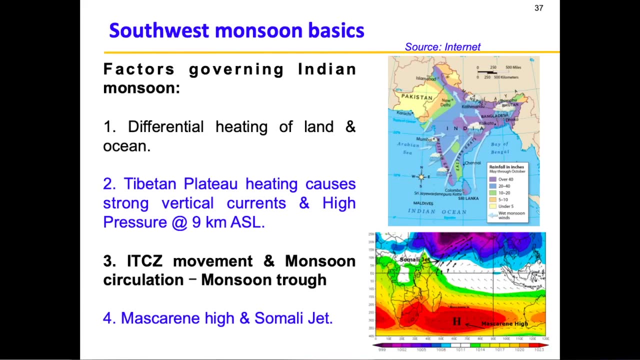 widespread heavy precipitation for a longer period of time, wherein you will get 100 mm or 150 mm in like seven or eight hours. that's why vortex is very, um tricky. okay, all right. so that brings me back to the last model, which is the southwest monsoon. um, like i said, the southwest monsoon is 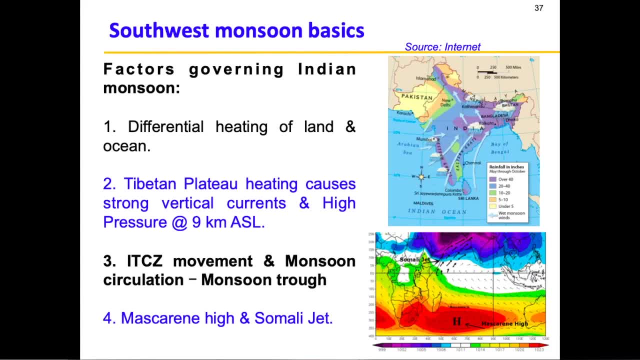 governed by many factors, which one is the differential heating of land and ocean. then you have the tibetan plateau, which actually heats up, uh, pulls the itcz up, so that itcz, which is the intertropical conversion zone, settles. near foot is the near the himalayan region and along with that you also have something known as a monsoon. 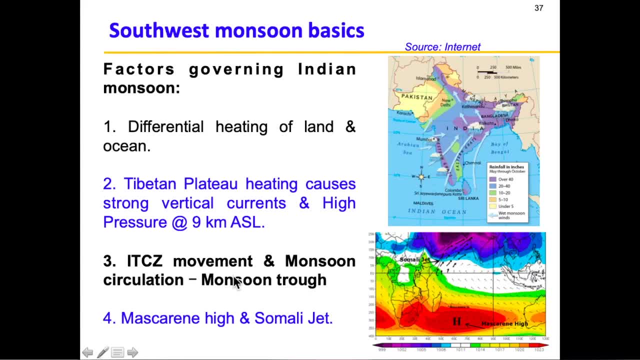 circulation, and these two put together is what they call monsoon trough, and then you have maskaran high, which is the high pressure in the southern indian ocean, which actually puts, which actually deflects the winds, and then that's how you actually have the somali jet formation, which 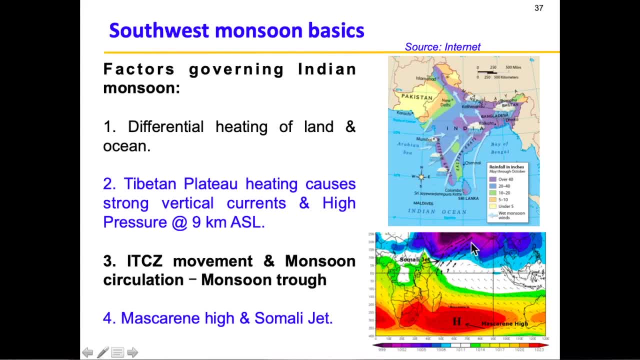 brings a lot of moisture to the in to the central part and western parts of india, and actually it brings a lot of moisture throughout the indian subcontinent. so i'll take a minute to explain what is this monsoon trough, because it's a very, very tricky. 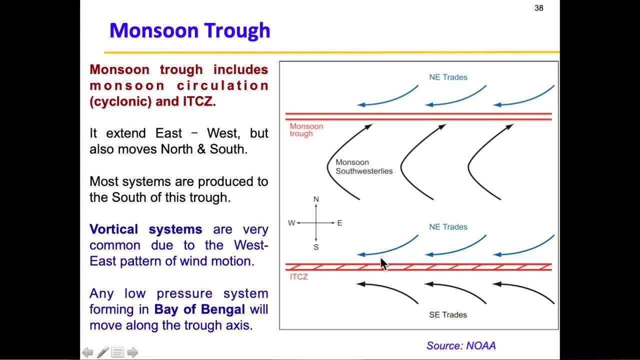 term, so monsoon trough. so you have itcz during normal time, but during monsoon what you have is your monsoon, you have itcz, which is this line. plus you have a cyclone, you have a cyclonic circulation which is very active, and that is what is known as the monsoon trough. monsoon trough embeds. 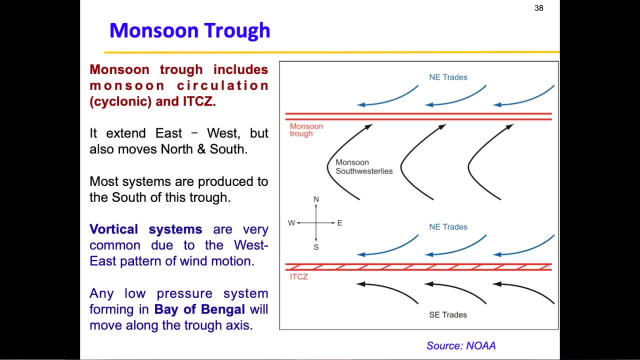 both the itcz and the circulation which is cyclonic circulation. and how does that cyclonic circulation come into picture? that cyclonic circulation actually comes from the middle of the mountain to picture because of the west east movement of winds. so you have the westerly winds, which are 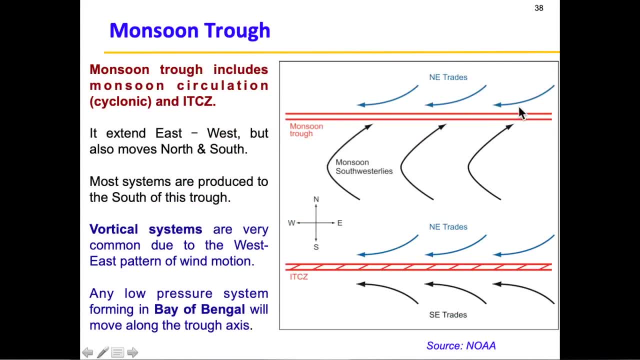 moving from the arabian sea and then, above that, you, you have these easterly winds because the hidley cell has moved up, so you have this easterly winds. so, if you see it, if you look at this, it actually automatically forms a cyclonic circulation, right. so east motion and west. 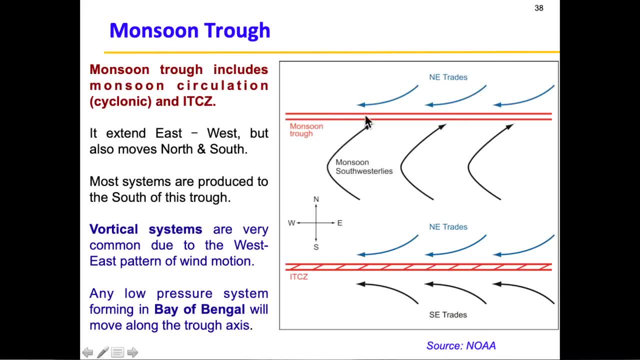 motion, east motion, west motion. so it's a, it's a, it automatically forms a, forms a cyclonic circulation, winds, which is which is known as the monsoon circulation. so the monsoon circulation plus the trough put together is known as the sorry monsoon circulation. 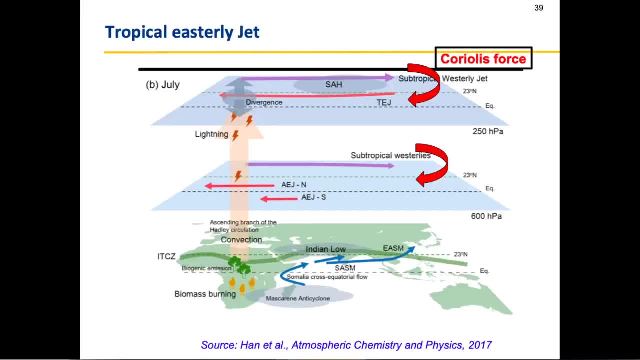 plus, the ITCZ is what is known as the monsoon trough. so this again just tells you that entire thing- ITCZ, moving up across equatorial flow, brings the Somali jet and that Somali jet brings westerly winds. and above this ITCZ line, 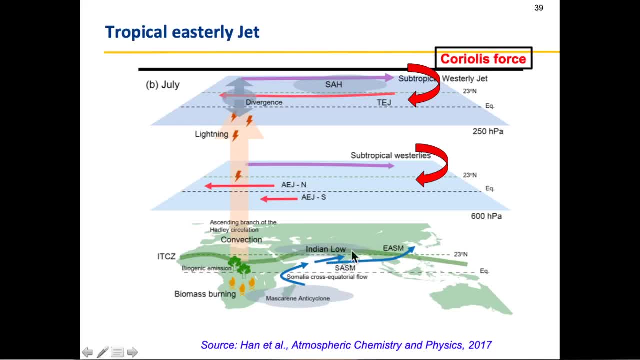 you have the easterly winds, and wherever the two winds meet, you have an active cyclonic circulation of monsoon, and that active cyclonic circulation of monsoon is what creates. so you have this. you have the cyclonic wind pattern which creates this monsoon circulation, and that is what dumps lot of that is. 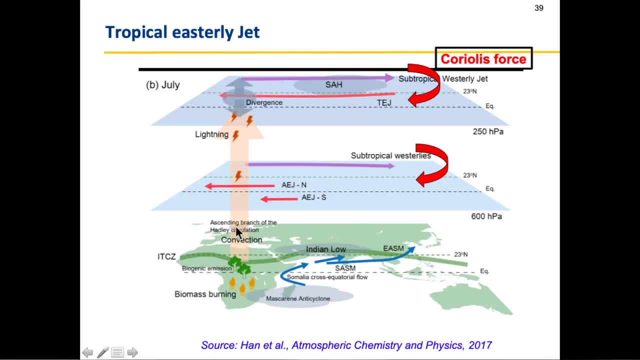 what keeps the monsoon alive for almost three months. and the role of Hadley cell is also highlighted here, because unless and until the Hadley cell moves to the north, you don't have the ITCZ shifting up. so this is the circulation that I was. 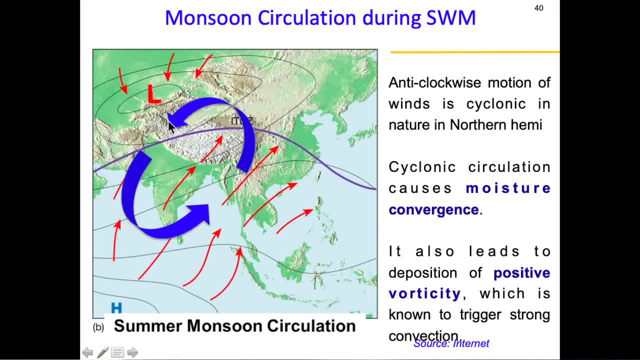 talking about this is the. so you have the westerly winds and you have the easterly winds, so, as the as they, as they, as they keep moving, you have the cyclonic circulation that creates in the northern hemisphere, and that, plus ITCZ, is what is known as the. 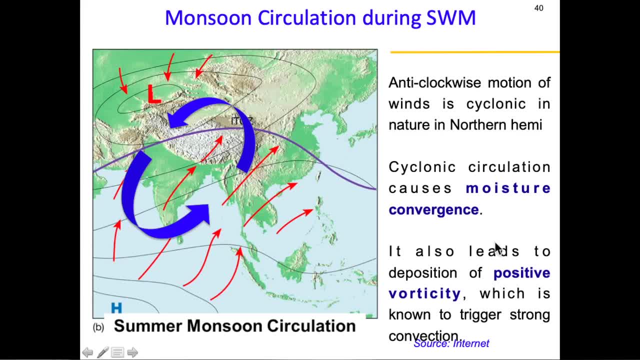 monsoon trough. the circulation is very important because it keeps the vorticity deposition aligned. so the unless and until you have the cyclonic circulation, you cannot have this vorticity gets, that gets deposited. and the second thing is you will not have any systems forming either in Bay of Bengal or Arabian Sea. 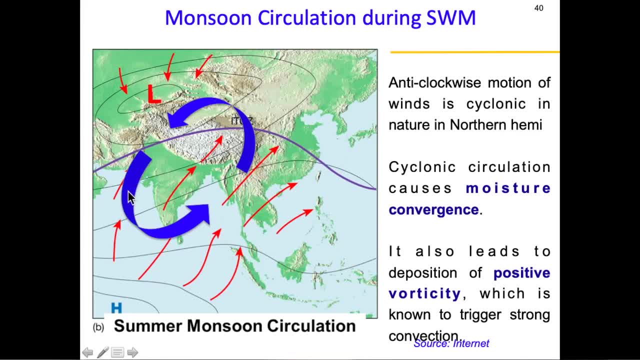 the reason. the cycling circulation ensures that during monsoon season you have at least 10 to 14 days of cyclonic circulation. that creates this vorticity. none of theseemonsoon troughs exist. they only exist in ten to fourteen good systems performing, which will move along the axis of monsoon trough. 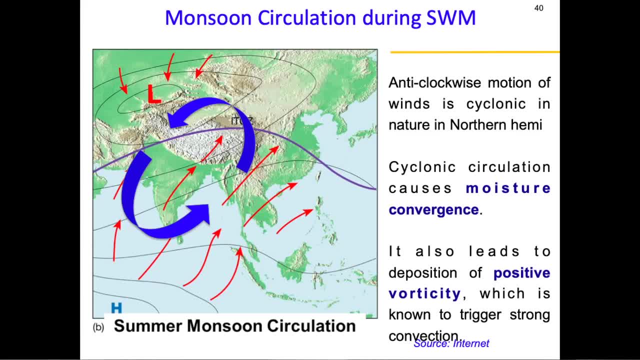 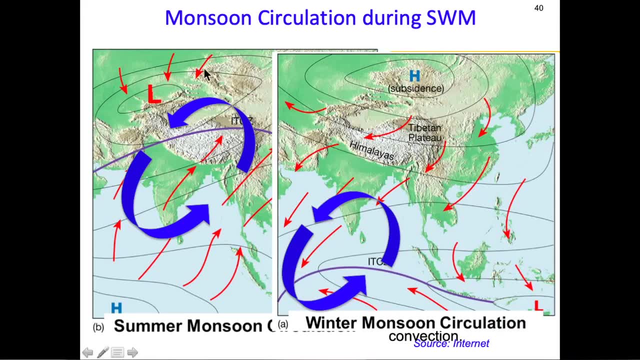 and they will dump lot of rain and that's why Southwest monsoon season you almost have a 8-89 mm of rainfall throughout the country, which is massive. so these are the specific features and during the northeast monsoon, ITCZ shifts down the cyclonic circulation also. 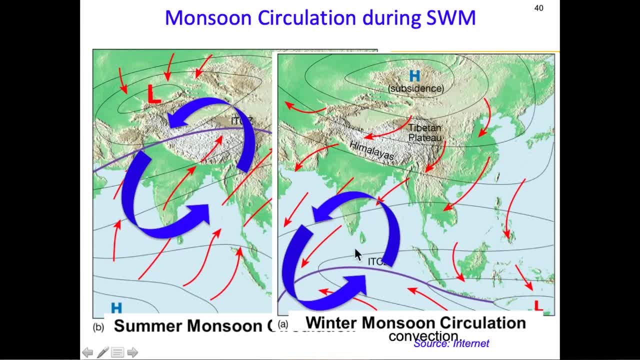 shifts down only active in the southern part of India, and that is and the as the southwest. when has? the South are the easiest moon transitions to northeastern most are difr? esoate for運 as the como? res? lun to northeast monsoon. the system, the, the cyclonic circulation systems become weak, and that's why 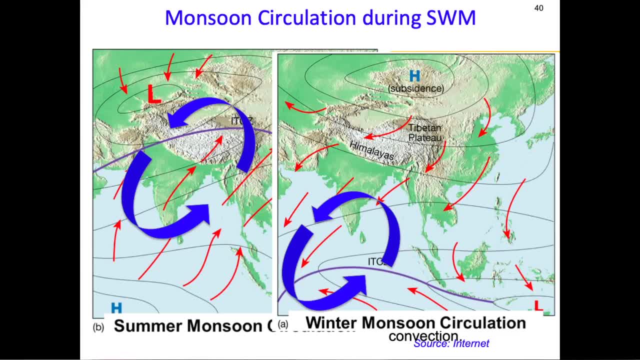 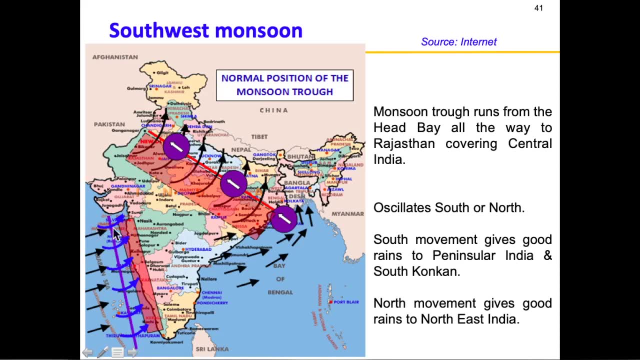 northeast monsoon doesn't give as bountiful rain as southwest monsoon. okay, so, like i said, this is the offshore trough. the offshore trough is the tipping pattern of winds on cyclonic movement of winds as the winds approach the western part of india. as they approach the western part of india. 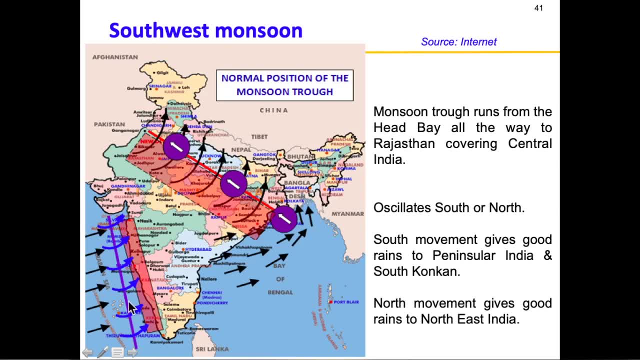 they. they deposit a lot of cyclonic vorticity in this region and the strong westerly winds from arabian sea they push these, so there is a cloud band formation along this line and these strong westerlies actually push these cloud bands towards the western parts of india, triggering 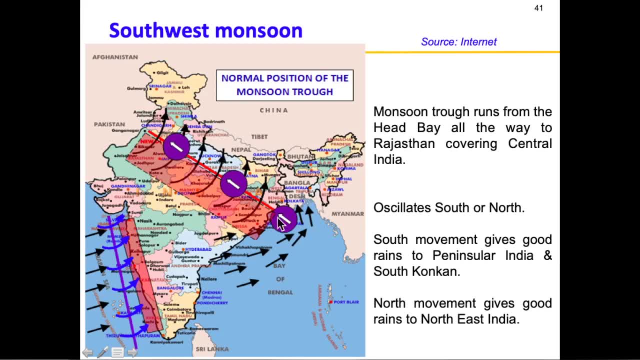 heavy to very heavy or extremely heavy rainfall episodes, and then any system that forms in Béxar Bengal will move. this is the monsoon trough, so this offshore drop, which is different, this is a monsoon truck which embeds the itcz plus the monsoon circulation, so any system that forms 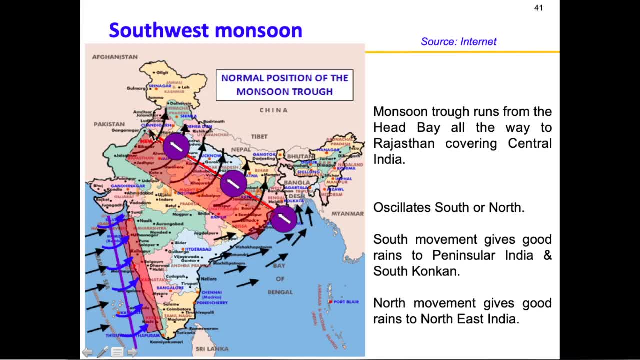 in Béxar, Bengal, will actually move along the line of itcz and, sorry, along the line of monsoon trough and this monsoon on the region of transport and otherwise. all these, those tons live in some way and survive, 스타 wanting to make land markets if they become a long distance or a dicenal to complete sense. 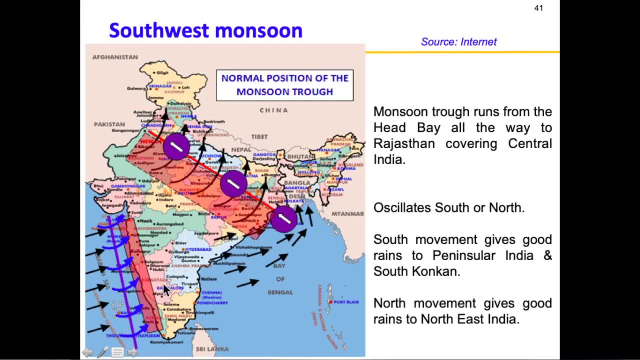 monsoon trough is not stationary. it moves up and down. so it moves. sometimes it is south, sometimes it is north. when it moves to south, then Kerala gets very heavy rainfall floods, like situation when it is in this region, in the central part of India. that's when Mumbai 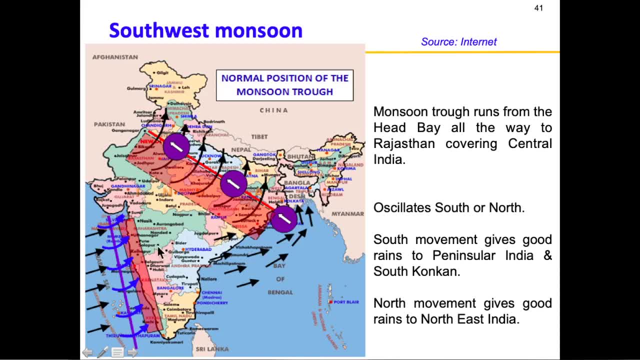 gets flooding type of rains, including Gujarat and also parts of Madhya, Maharashtra and sometimes even Hyderabad, like Telangana places as well, and when it is north of, when it moves north, then Uttar Pradesh and northeast India and Nepal- all these places get a lot of floods. 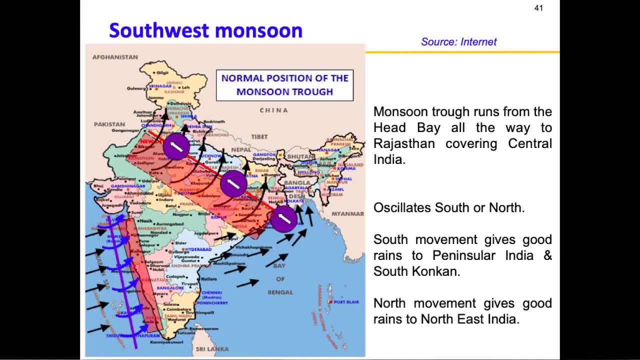 so this movement of monsoon trough is very, very, very important feature of monsoon and lot can be said by just by tracking this monsoon trough. and it is always slanted, it is never straight. the reason it is slanted is because of the effect of Coriolis force. so this monsoon 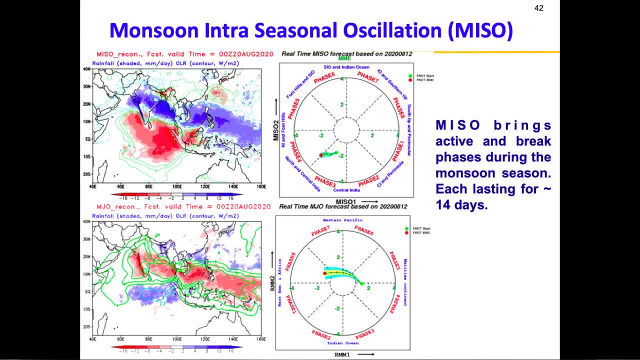 trough, which is also known as monsoon intra-season oscillation, can actually be found through models. there is an active IITM model, Indian Institute of Tropical Meteorology, which is tracks the meso how it moves, how the monsoon trough moves during the monsoon season up. 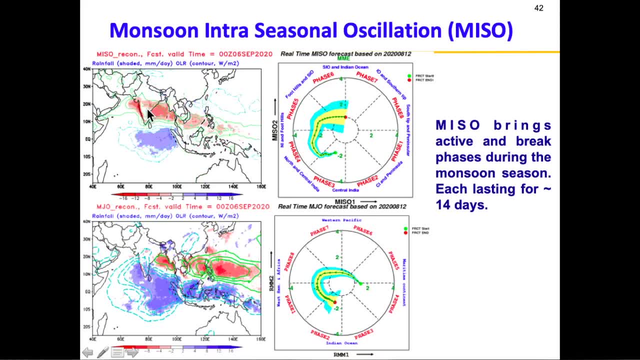 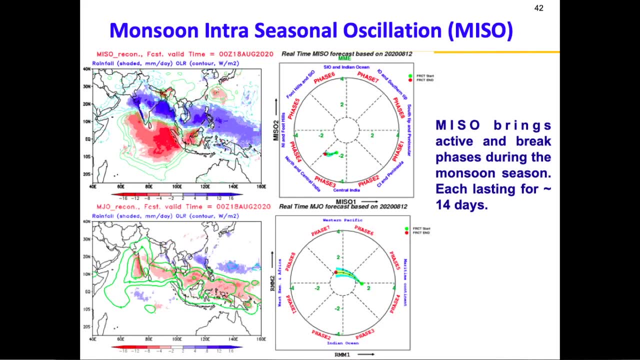 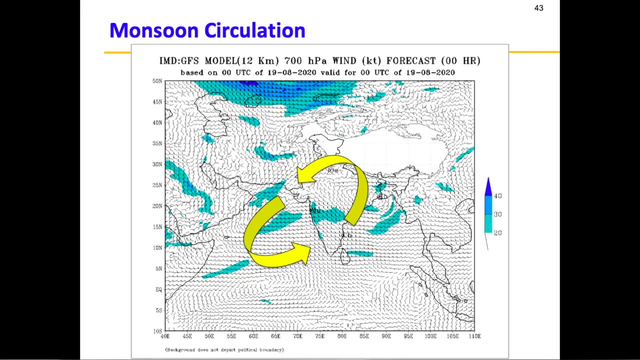 and down, up and down north and south. okay, and I mean, lot of things can be actually known, but this, this is just a guideline why it doesn't. a lot of issues associated with exactly tracking the monsoon trough, but still it is some guidance. this is that monsoon circulation cell that 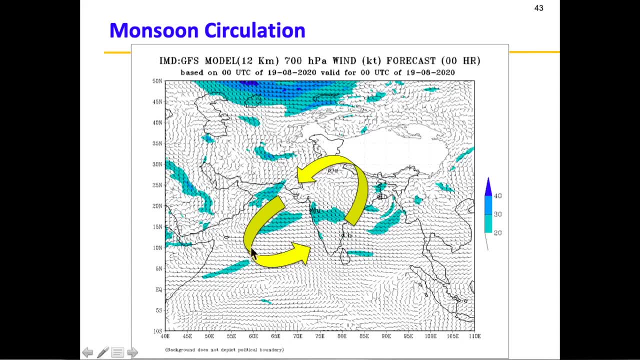 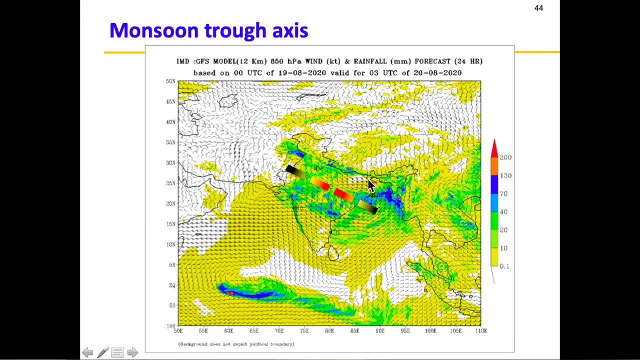 I was talking about. you can clearly see a distinct circulation cell which is covering entire India and giving widespread rain. this is the monsoon trough axis. monsoon trough axis is where the westerly winds and the easterly winds meet, so this is the westerly motion, this is the 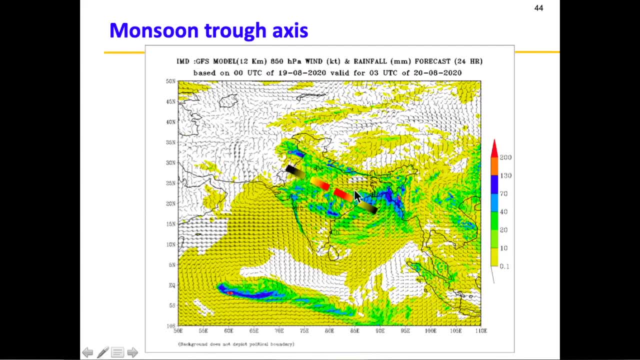 easterly motion. so wherever they meet, that's where the monsoon trough forms. and this system, this which has formed in way of Bengal, will actually move along the monsoon trough axis all the way from way of Bengal to western Rajasthan, dumping lot of rain, mostly below. 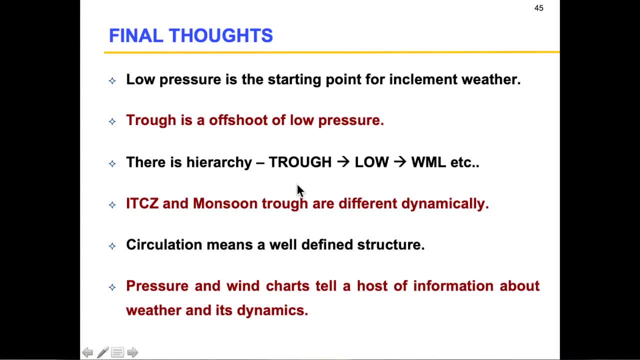 the axis of monsoon trough. all right, so this is bringing me to the last slide, which is my final thought. low pressure is the starting point for implement weather. so hierarchy and all these low pressure actually start from the wind, movement and the pressure. how the pressure behaves: wind and pressure. moisture is automatically coming from the 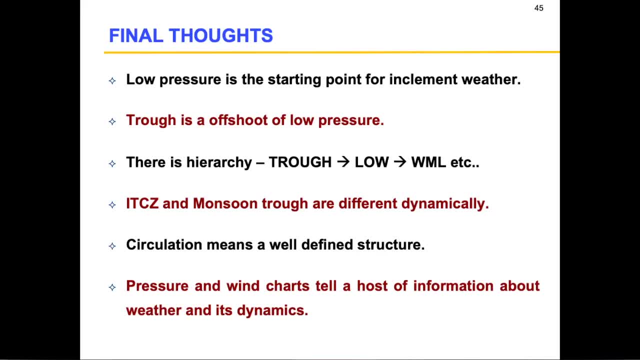 ocean. no problems there. but low pressure is the starting point and you have different offshoots of low pressure, like trough. you have vortex, you have well marked low and everything but low pressure or cyclonic system is something which is a starting point. cyclonic system is a very broad term. low is a specific term. trough is a very broad term. low is a starting. 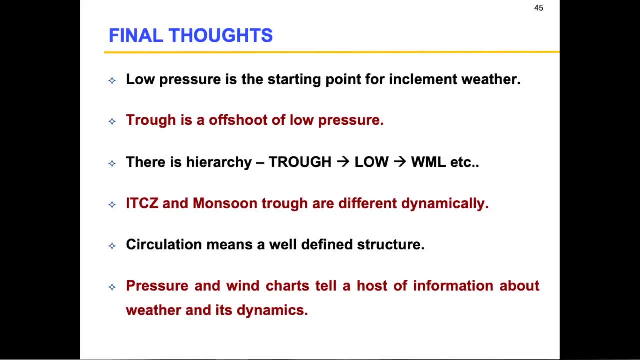 monsoon trough is a specific term. windmark is a specific term. ITCZ and monsoon trough are dynamically different because monsoon trough actually embeds ITCZ and the monsoon circulation. distinct monsoon circulation, cell Circulation, means a well-defined structure. 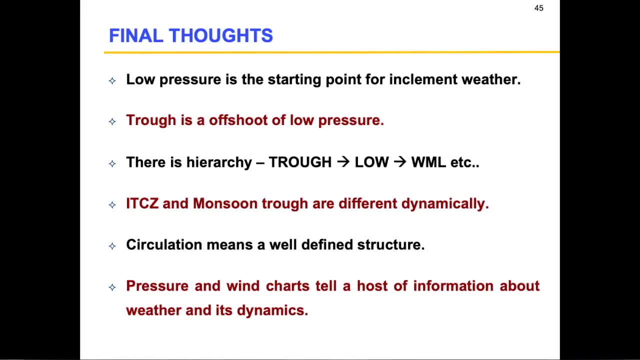 Pressure and wind chart actually tell a lot of information about weather and its dynamics, and temperature is important, but pressure and wind charts are the ones which actually have not a host of information, and these are actually important for moisture convergence. We always look at the output, but I feel like we should always take one step back and instead 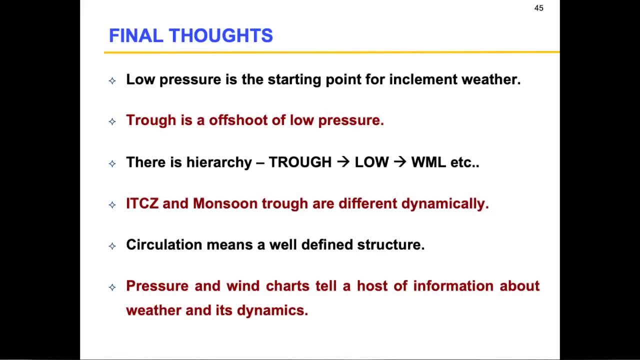 of saying that moisture has converged, we should actually see why that moisture has converged in that location and that actually can only come out from dynamics, which is looking at wind charts, pressure charts and looking at basics of convection, momentum and this Coriolis force and all these things that I talked about. A lot of details is in the basics. 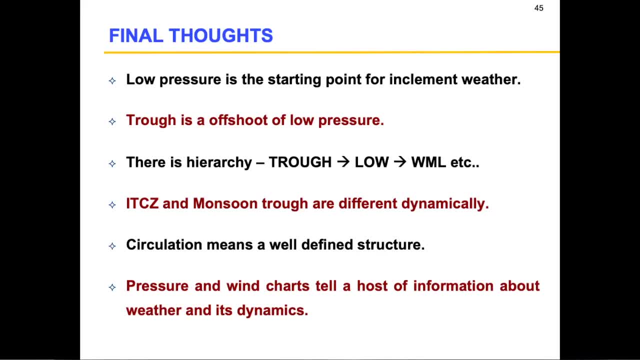 so that's why I thought I will make this video. Those who are interested can take up a lot of things from this video and, of course, this is not the only video which is available. There is a lot of information available over internet. there are a lot of books, a lot of other nice videos which are available. so 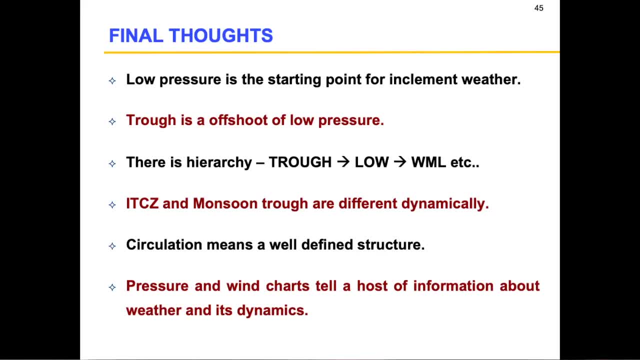 you are free to look at any of them, but I just wanted to make this video to give you the basics of weather dynamics, which is of interest to me. So thank you so much for watching this video and please subscribe to this channel. I know it is a long video, but I hope it is.